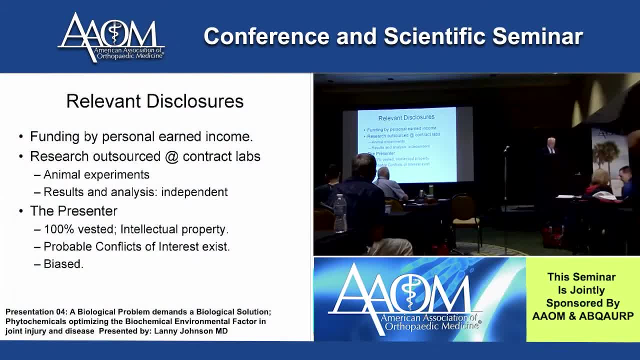 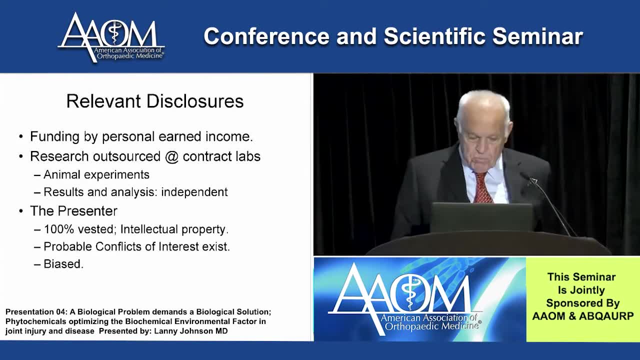 Okay, thank you for the opportunity to be here again. I learned a great deal by being here, and so I'm very appreciative. All of my disclosures are on the AAOS website, but generally you should know that I do have a lot of conflicts of interest in what I'm showing you and I'm very biased. 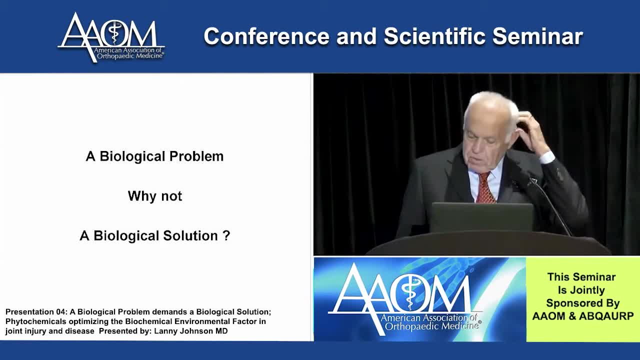 So, actually hearing the meeting as it's been going on, I reshaped my talk a little bit so that I could address a number of issues that have been discussed here, But basically my issue is that we have a biological problem and somehow why not have a biological solution? 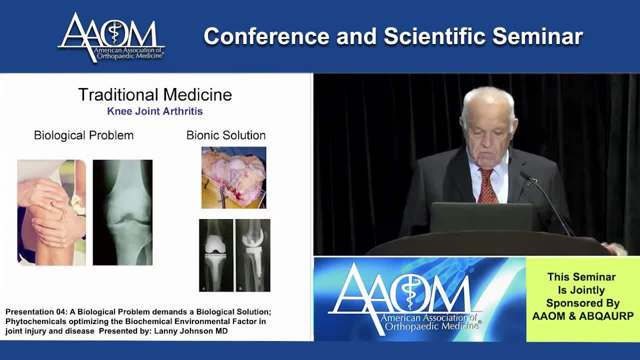 So what we find out in the knee, for instance, if somebody has a biological problem, we're going to treat this type of problem with a rather large incision and then put in metal and plastic, and now we have a bionic solution. 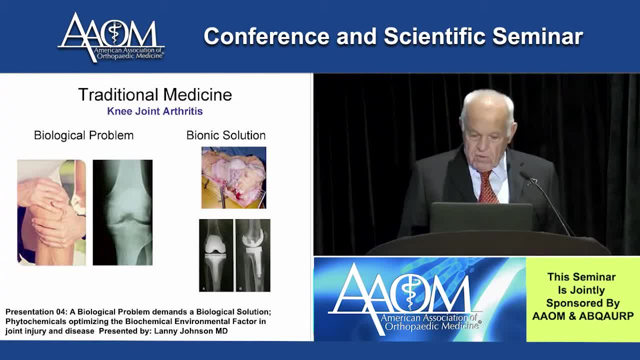 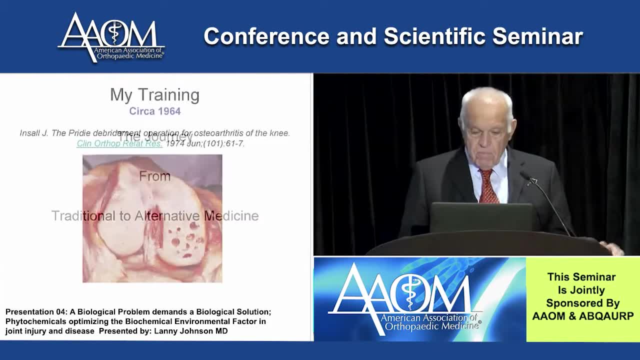 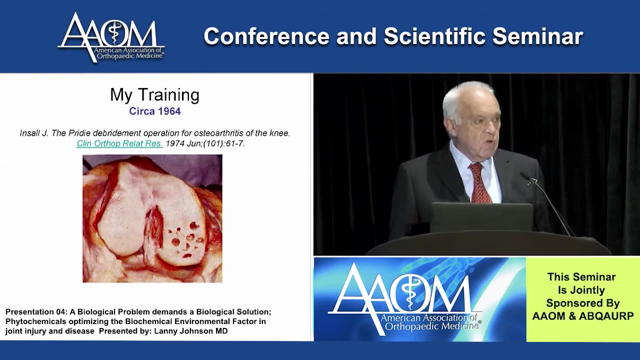 And although they're satisfactory in most situations, I don't think that's exactly where we should be going. So, So, over time, I've had a journey from traditional medicine to alternative medicine, and in my training, this is the way I was told that we needed to treat people that had some arthritic change on the inside of their knee. 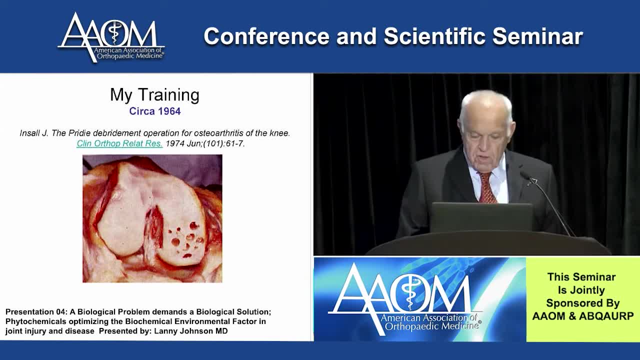 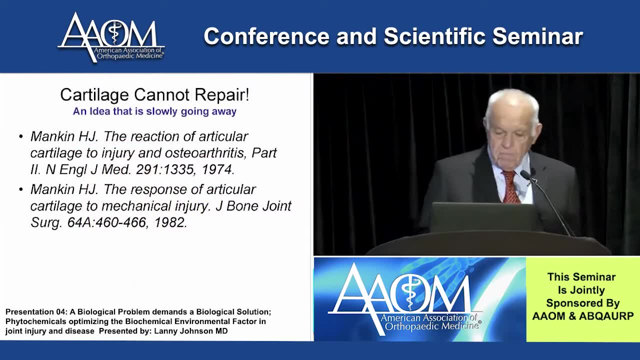 And of course you can see that the treatment was far worse than the condition, and this was called a pretty procedure, which really wasn't very pretty. So then we knew for certain that the cartilage could not repair. That was not too long ago. 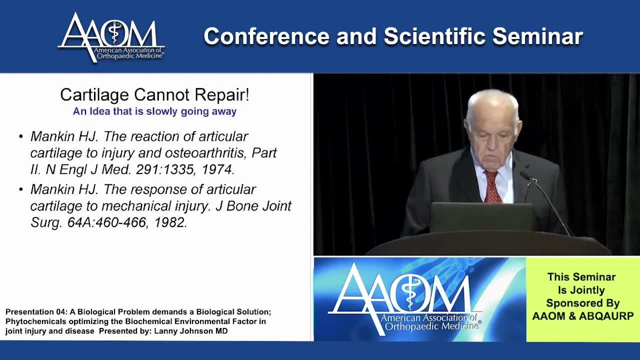 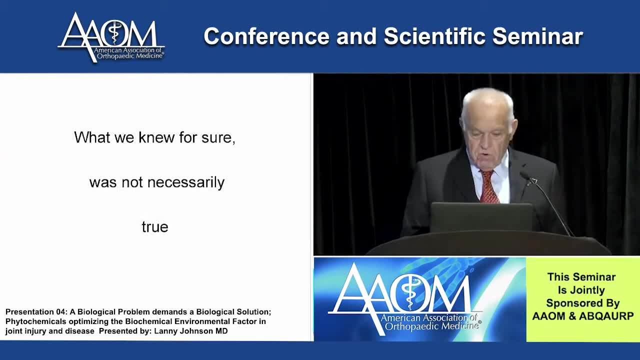 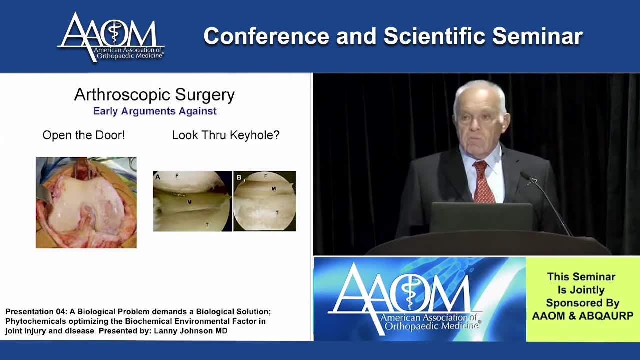 But that idea slowly going away. So the more famous the person that was certain that of this edict. that seemed to change over time. So what we knew for sure was not necessarily true. But then when arthroscopy came along, it was interesting that the group that was most against it in orthopedic surgery was the sports medicine doctors of the day. 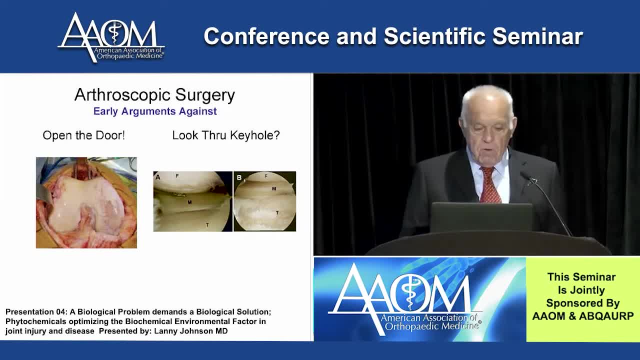 And of course you can see that's changed. And they would argue: why wouldn't you allow us to open the door rather than look through a keyhole? And I used to tell them that well, gentlemen, we could go out on the street and ask people: why wouldn't you allow us to open the door rather than look through a keyhole? 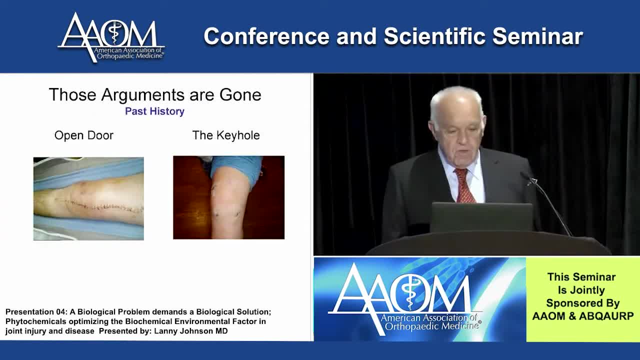 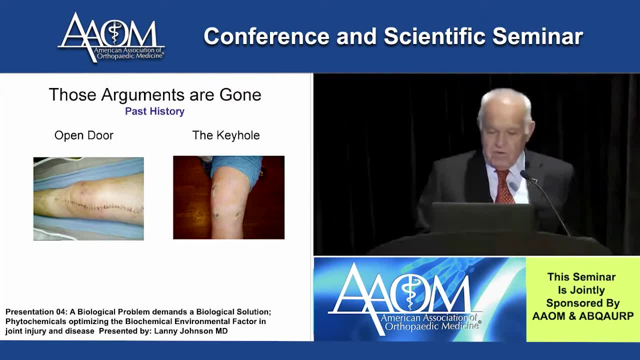 And they would say, well, what they'd like to have done. And so here we see, the arguments are long gone, This is past history. You can see the incision from opening the door And you can see the incisions that happened, the minimal trauma from looking arthroscopically through a keyhole. 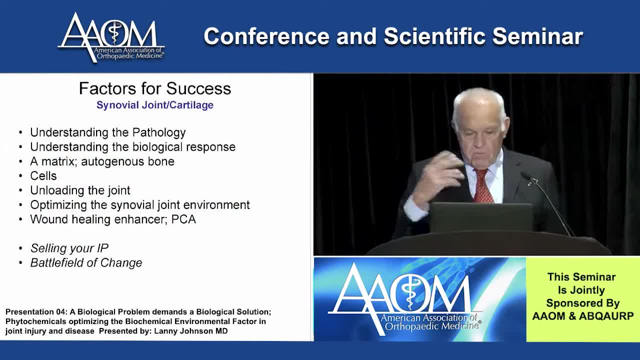 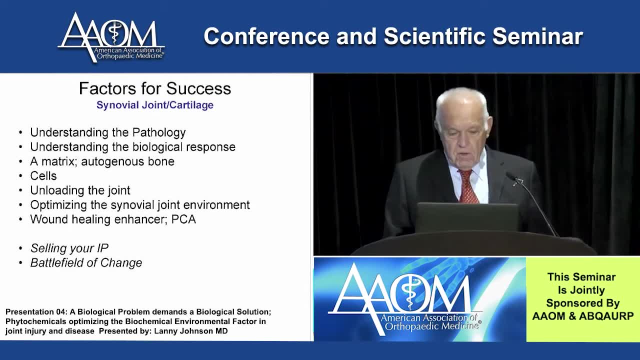 So what I wanted to do- and I've reshaped this somewhat because of having the opportunity to sit at the whole meeting- I wanted to discuss understanding the pathology behind end-stage osteoarthritis, understanding the biological, The biological response, the fact that we need the ingredients of the matrix cells. 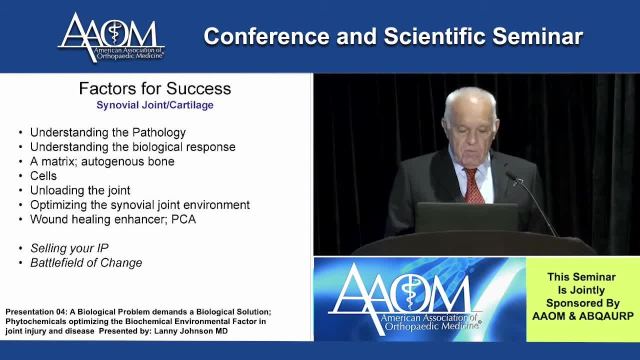 You'll be amazed at what I'm going to show you about unloading the joint, And then we'll talk about optimizing the synovial joint environment, And then, finally, a wound healing enhancer, And, if I have time, I'll deal with selling your intellectual property and how you deal with the battlefield of change which you're in the middle of. 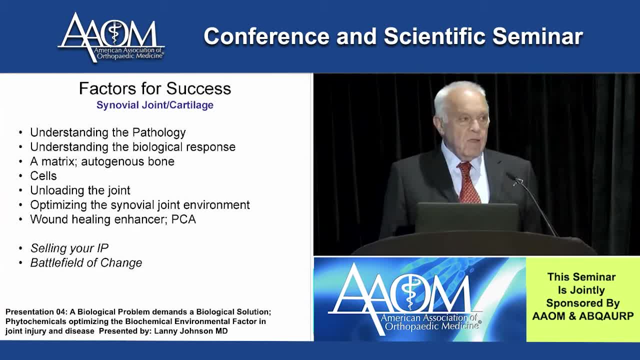 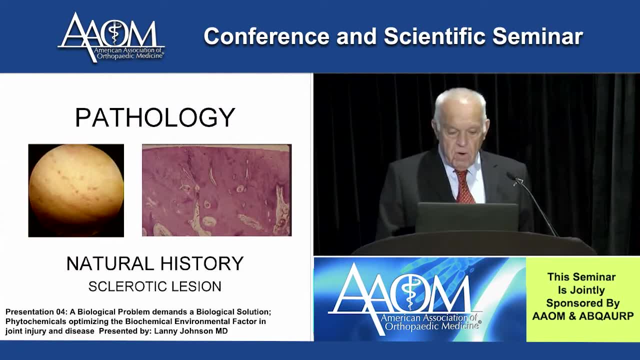 And if I don't get to that in the interest of everybody's time, I've written that up already at the end of what I wrote for you. So let's look at the end-stage osteoarthritic sclerotic lesion And the natural history is that the cartilage gets worn off and there are dead osteons on the surface. 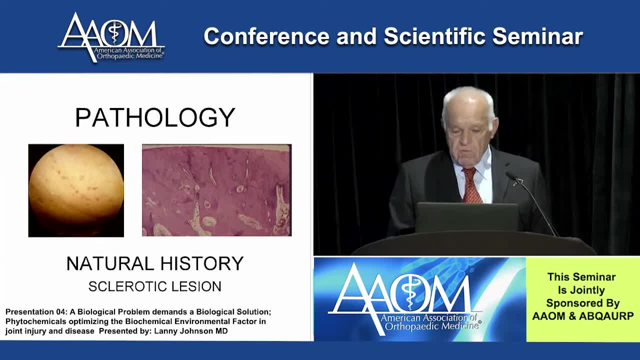 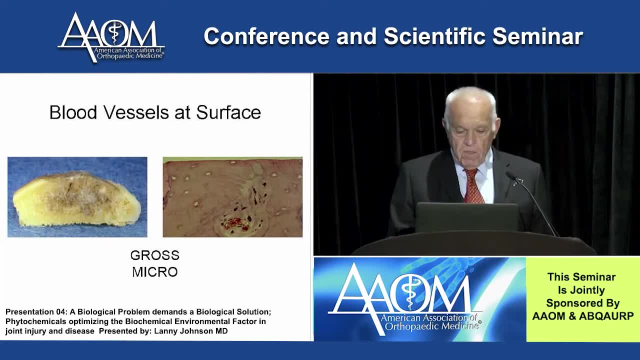 but the blood supply is starting to come up near the surface, as you can see by those fissures. And here you can see the blood supply is actually right at the surface, even though there was an injury and wore the cartilage all off. 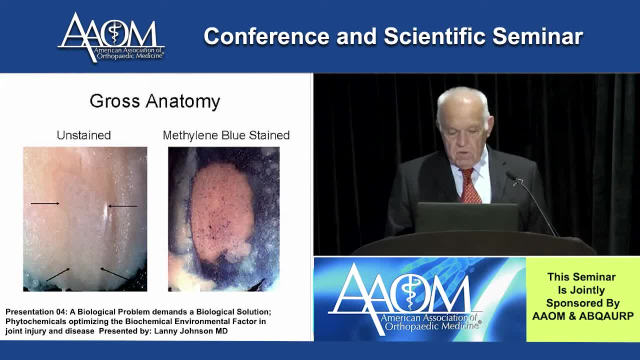 And so if we look at the, If we look at the gross anatomy, unstained, we'll see that it just looks like a shiny mirror-looking surface. but if we put methylene blue on it, we'll see there's a number of pits. 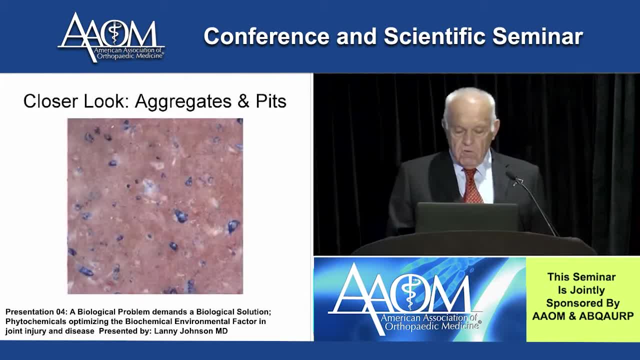 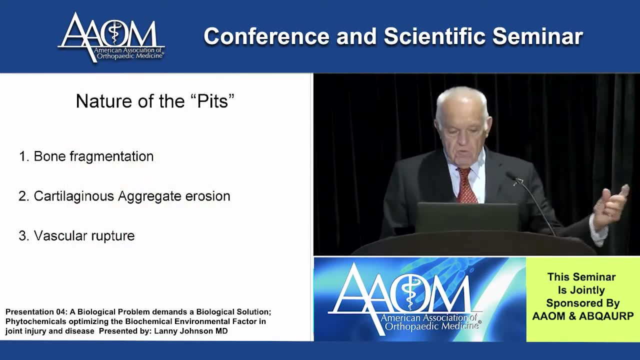 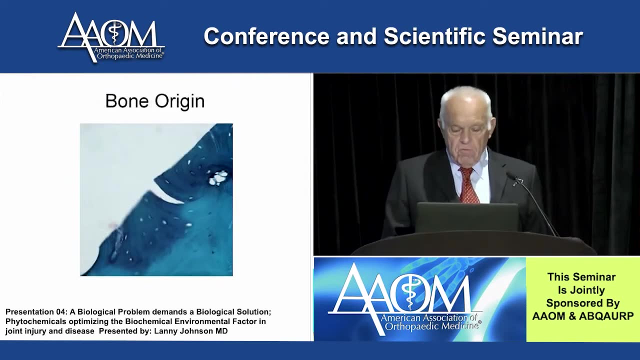 And we published this in the NEED journal. A closer look shows that what we have there is aggregates of cartilage and multiple pits, And the pits are of three natures: bone fragmentation, cartilage aggregate erosion and vascular rupture. There is one of the fissures that occur from bone origin. 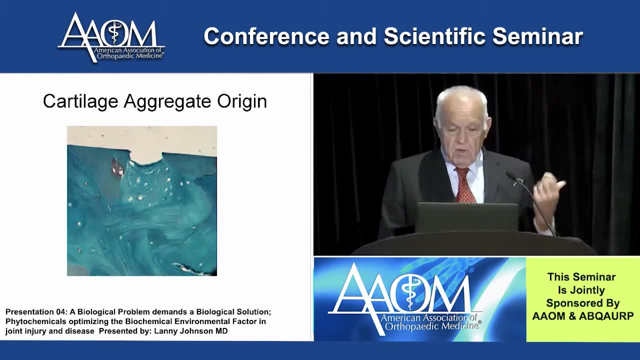 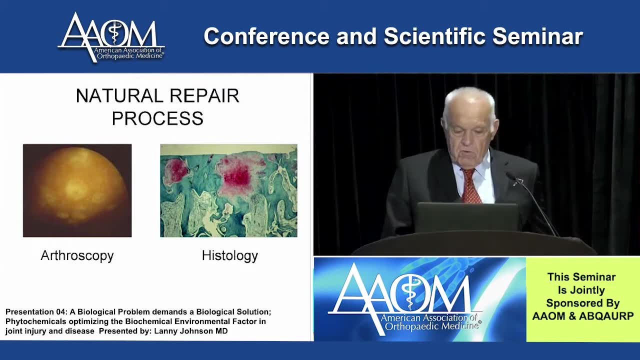 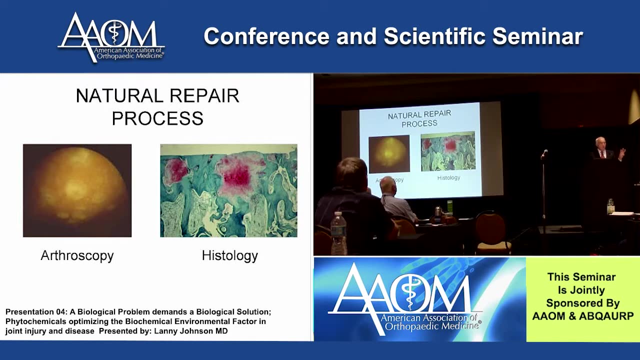 And here's a cartilage, A cartilage lesion, a regrowth that has eroded. And the other one would be vascular- That didn't show up, Sorry- And the other one would be where blood vessels ruptured. So those three pits all serve as a home for cellular treatment. 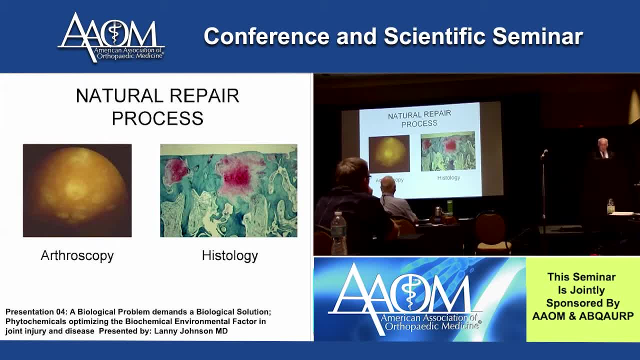 So if you can think about that, that is an opportunity. But this is what's probably going to be important for you to clearly understand, and that is when we look at these end-stage sclerotic lesions, there already are cartilage bundles, or we call them cartilaginous aggregates. 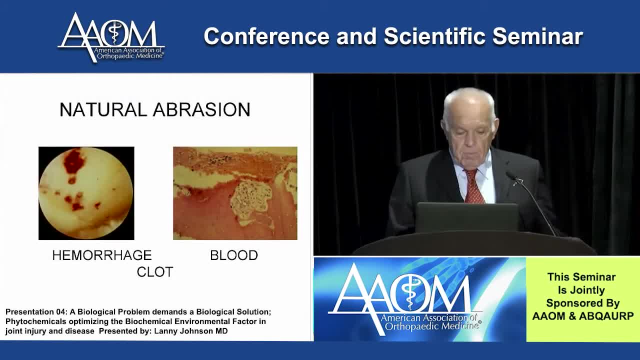 that are moving up towards the surface, And these probably happen. Here's a natural history of a patient who came who had an end-stage lesion. Arthroscopically. we can see that it bled and we can see the vessel at the surface and the bleeding that occurred there. 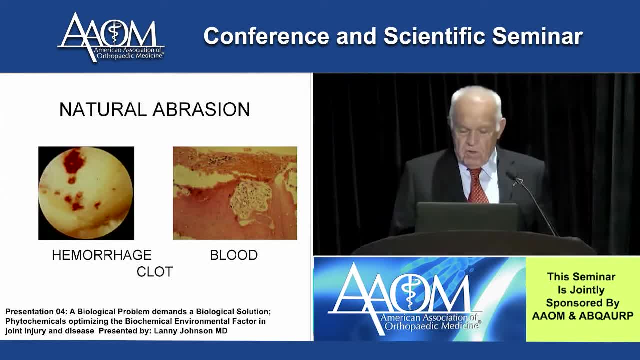 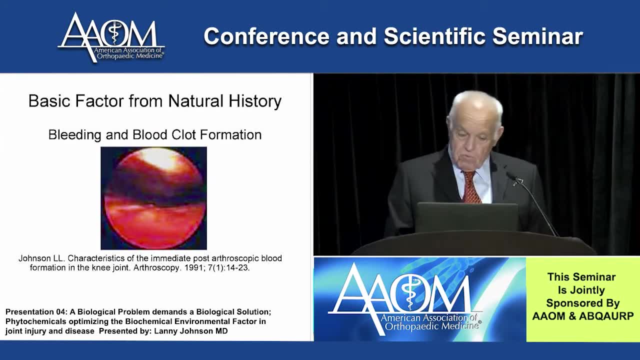 These may be- and I can't seem this longitudinally- may be one of the reasons there are aggregates. So we know one of the basic factors of healing is certainly, as you just learned, bleeding and blood clot formation. And what was interesting, that orthopedic surgeons doing arthroscopy didn't think that a blood clot formed. 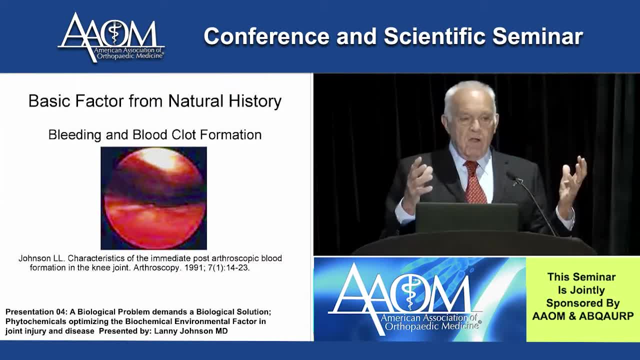 because they looked in with the scope, distended the joint, washed it all out and when they looked there was no bleeding. So what I did? I looked at 22 consecutive cases after I took the arthroscope out, waited 5 to 7 minutes, looked back in, washed it out. 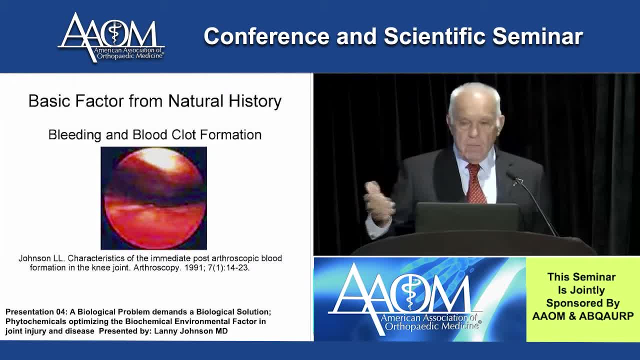 and every place there is a laceration or any incision, a blood clot forms on cartilage or on meniscus or on synovium, And for some reason the orthopedic surgeons were blind to the idea that a blood clot did work in the knee as well. 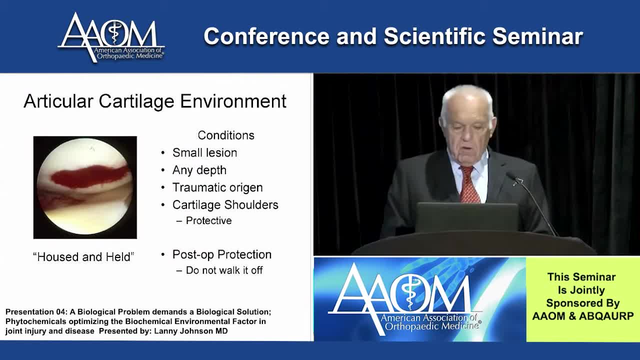 And so what we have is an articular cartilage environment. This is the type of clot you would see in a partial thickness lesion, And so this can be a small depth, It could be any depth, It could be full depth. This one is of a traumatic origin. 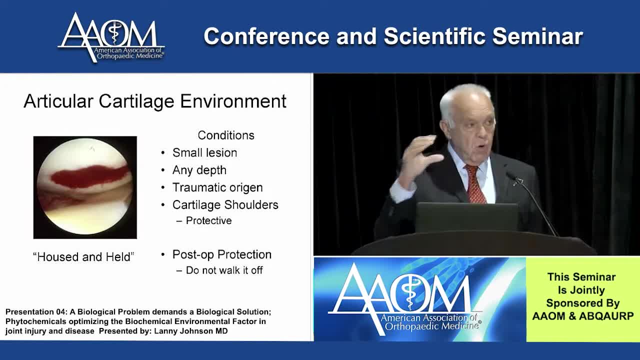 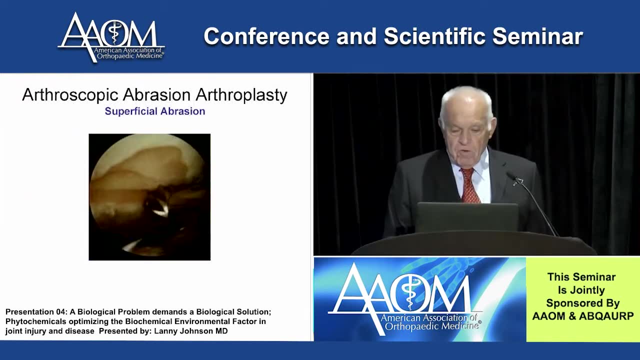 If they have shoulders on them so that you can house and hold the clot. there will be articular cartilage healing by subsequent biopsy. But what usually happens is the patient wants to get going right away, walks the blood clot off. So I had the idea a long time ago of arthroscopic abrasion arthroplasty. 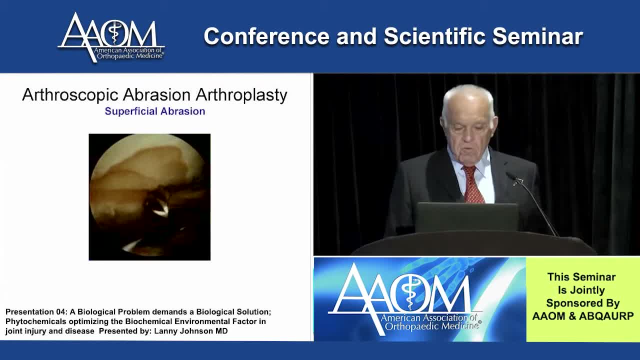 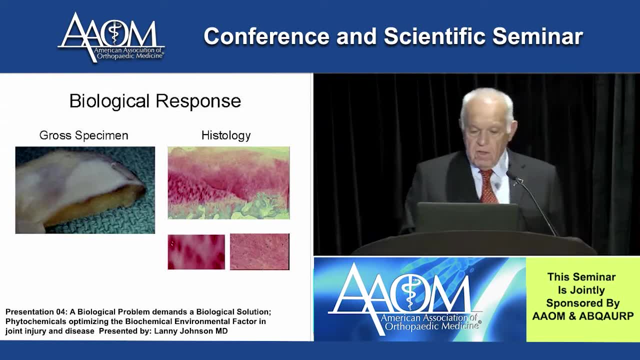 where it was a superficial abrasion like dermabrasion and exposed the superficial vessels. And then what happened after that was that there was a regeneration of the cartilage on the surface if this joint had been protected. You can see on the left lower side. 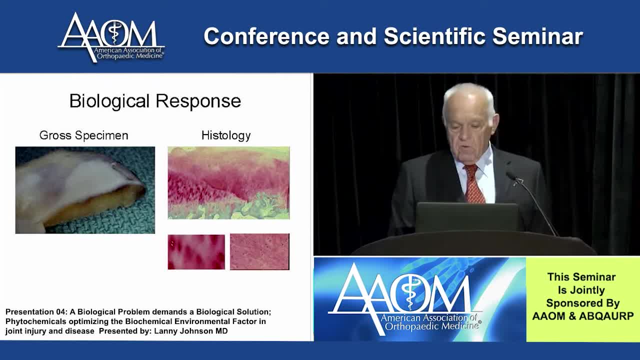 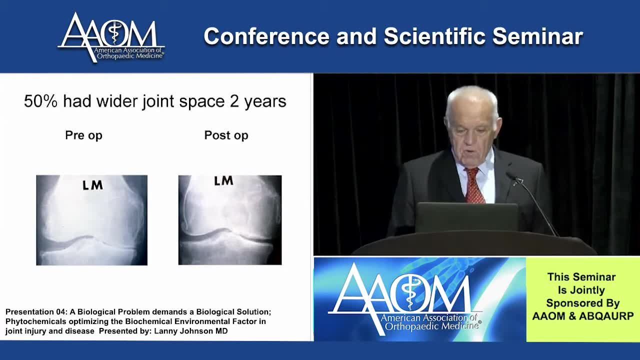 on the right of the histology you can see normal cartilage and then you can see the fibrocartilage to the right which is adhered perfectly to it, And of these patients about half had a wider joint space at the end of two years. 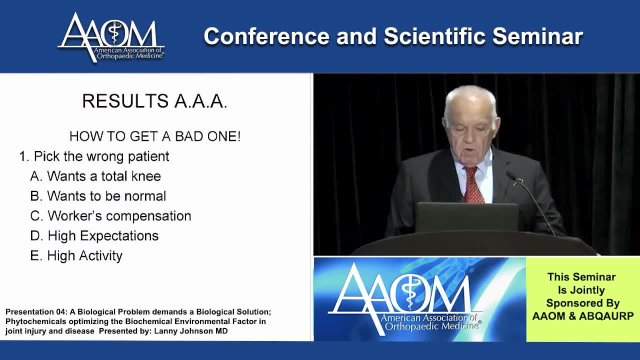 Not all, But what we learned over time was how people could get a bad result, And so they would pick the wrong patient. Somebody wanted total knee, Someone wants to be normal, a worker's comp, Or you can't meet their expectations. or they wanted to run the marathon. 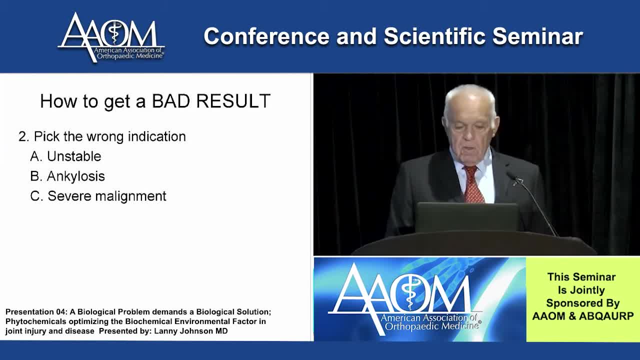 And you'd get a bad result. If you pick an unstable knee, an ankylosis knee or one with severe malalignment And the other way that's most common is that you'll cut too deep and you'll make a severe injury and the patient will hurt more. 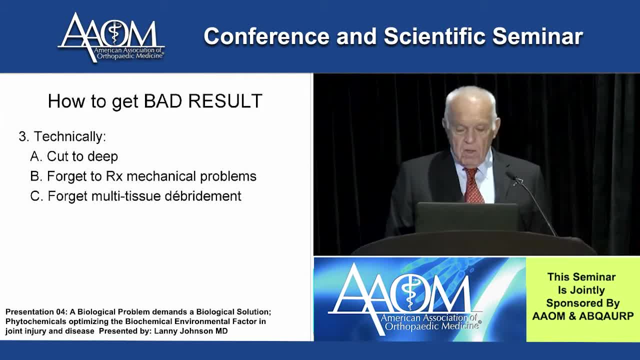 And then you forget to treat the mechanical problems, the misalignment, or you forget to debride other soft tissue problems, Or finally let the patient walk on it right away. They'll walk the blood clot off and there won't be any healing. 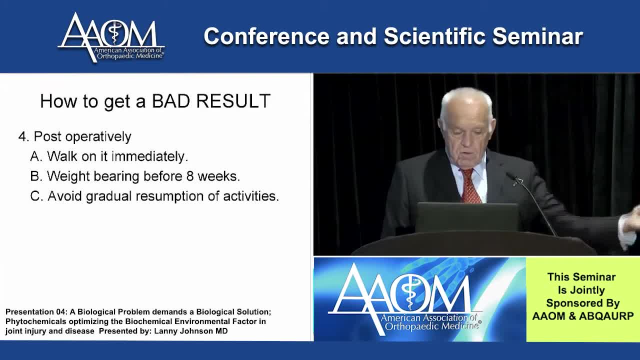 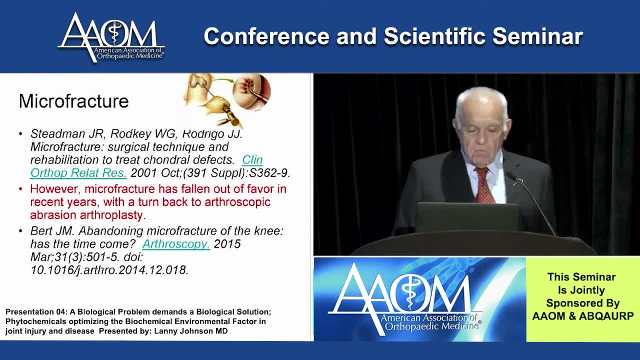 So normally these patients had to be protected, just as you would protect an incision on the arm Or elbow or hand for a number of weeks And then gradual resumption. So then, after this micro fracture became very, very popular, Stedman and Rodkey, both friends of mine. 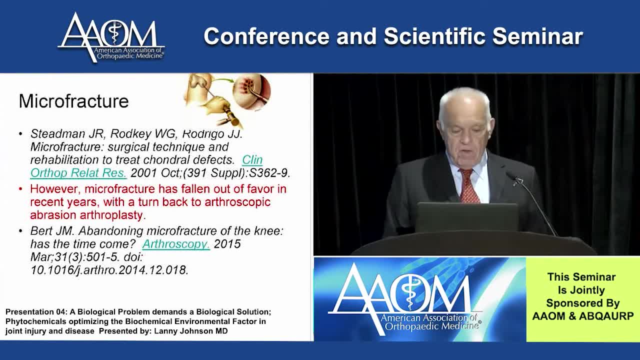 But, however, over the years now it's fallen out of favor, And Jack Burt last year, and others have now, have pointed out the failures of micro fracture and some of the different problems that it has caused, And so people have turned back, interestingly enough. 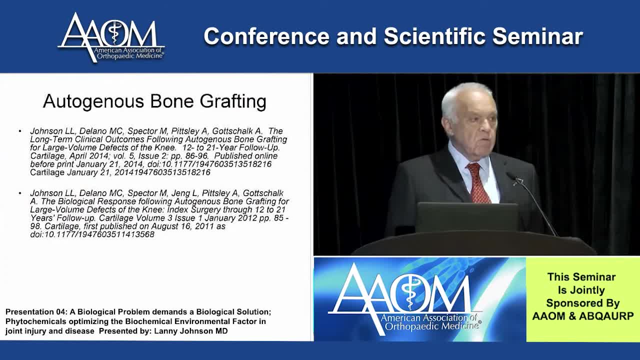 to abrasion arthroplasty. Now I want to share with you what are long-term follow-ups, And I think if you go 13 to 21 years, it should be a satisfactory long-term follow-up, And I published both of these in the cartilage journal. 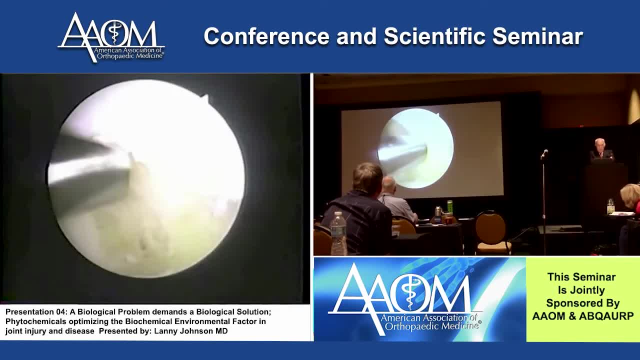 And this is the type of thing we did. We had lesions that were large-sized articular cartilage defects, of which we debrided arthroscopically, And then we used autogenous bone from the tibial metathesis proximal. 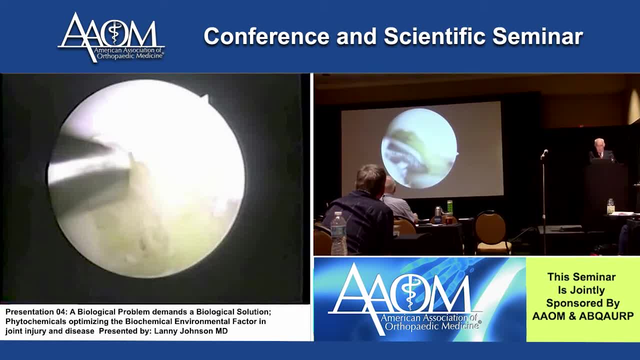 Put it in with a super diameter syringe, Picked it down in these patients, The ones we did arthroscopically- We allowed a blood clot to form And then the patients had to protect that for about eight weeks And then we had the opportunity to do second looks. 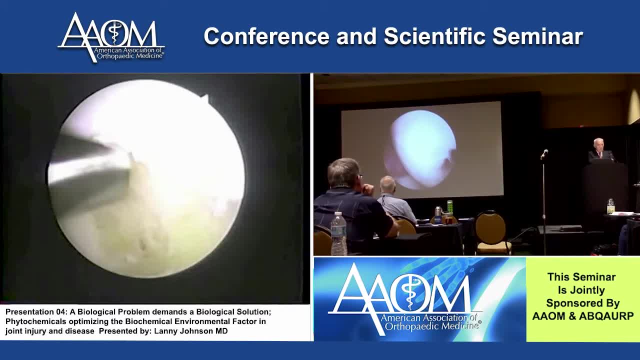 And this one happens to be two years later- of which there's the second look, A patient who's completely asymptomatic but granted a second look. Here is the core biopsy of this patient And it shows that there's still soft articular tissue but bone beneath. 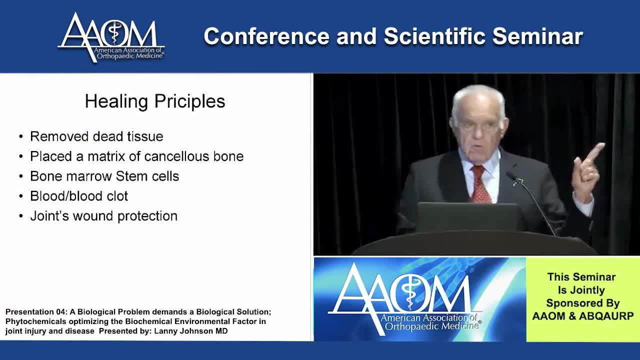 And one of the healing principles in this was we removed the dead tissue, Placed a matrix of cancellous bone, We had bone marrow- quote unquote- stem cells, We had blood and blood clot And then we protected the joint. Here's a patient that had a huge defect. 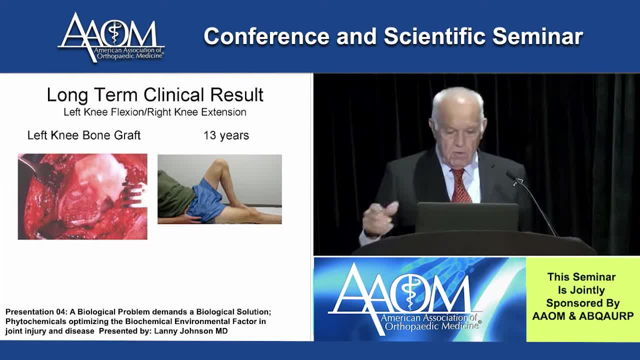 I got severely criticized for doing him because he had already had leukemia And with leukemia treatment had major loss of articular surface and large defects of his condyle Over to the right. you see his flexion of his left knee at 13 years. 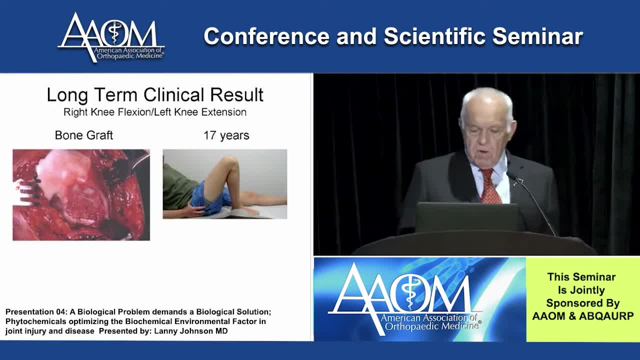 Extension of the right knee. And here you see flexion of the right knee and extension of the left knee at 17 years, Follow up on that knee. So I showed that these autogenous bone grafts, which meet all the criteria necessary for the regeneration of an articular surface. 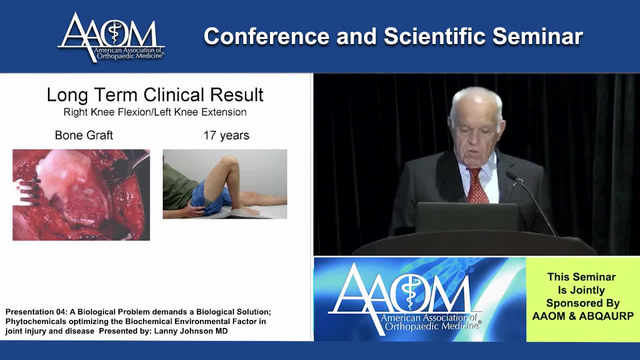 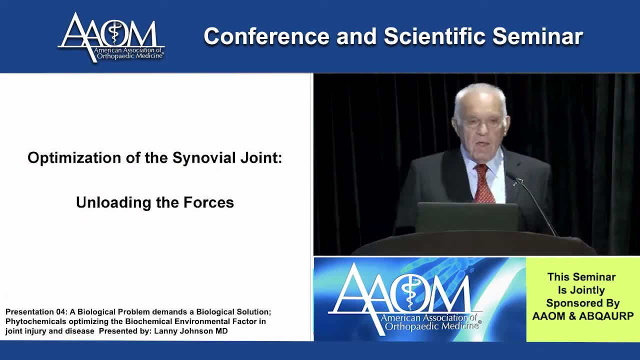 works, even in a very, very large lesion with long term follow ups. Now I'd like to show you something that has come across my attention recently, And this is truly amazing to me, Although I knew that if you did an osteotomy of the hip, 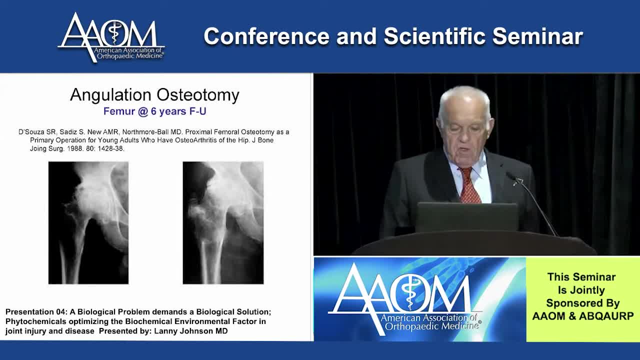 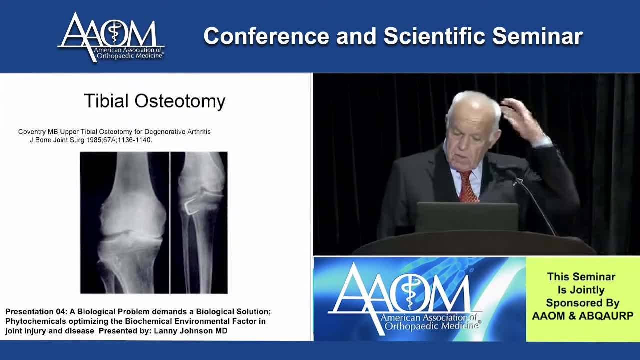 and the before on the left and the after on the right. if you change the angulation, there'd be a small joint space would occur. And then Coventry showed that if you did an osteotomy on the tibia, took a piece of bone out and realigned 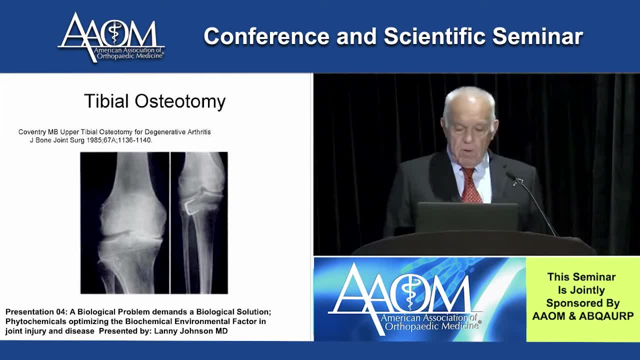 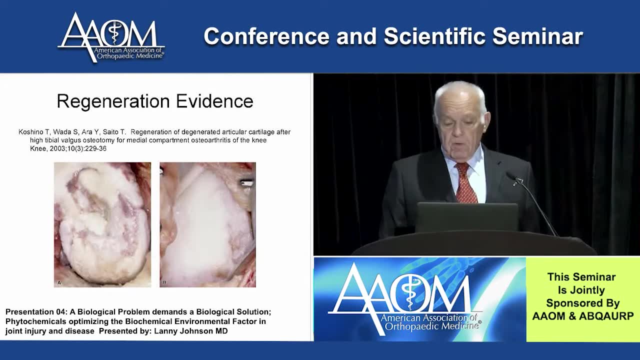 that there would be a wider joint space on the medial compartment. And then there's work done that was done arthroscopically before and after osteotomy to show a huge lesions in the knee journal and how it was healed afterwards. So I'm kind of surprised that they did two big open operations. 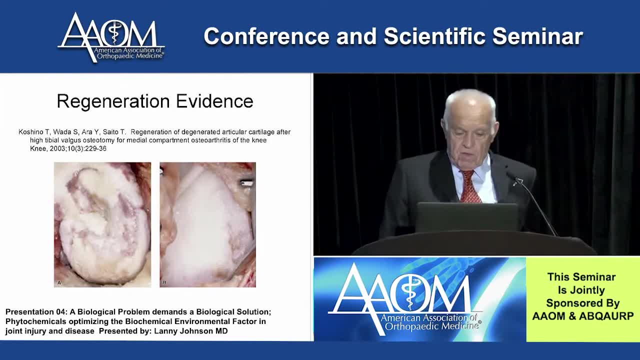 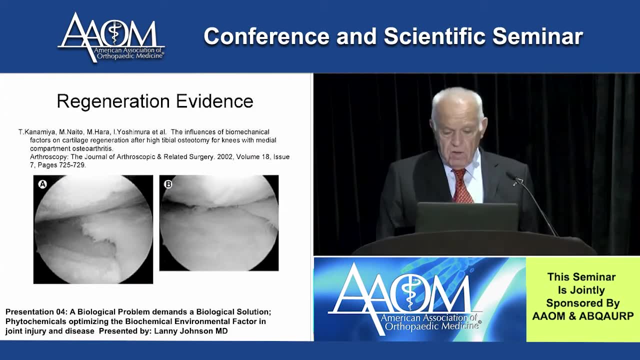 to get it. It was nice of them to be able to show us that. Then research was done that showed that arthroscopically here's a bone on bone in the joint osteotomy and then subsequently regeneration of the cartilage, So only unloading that medial compartment. 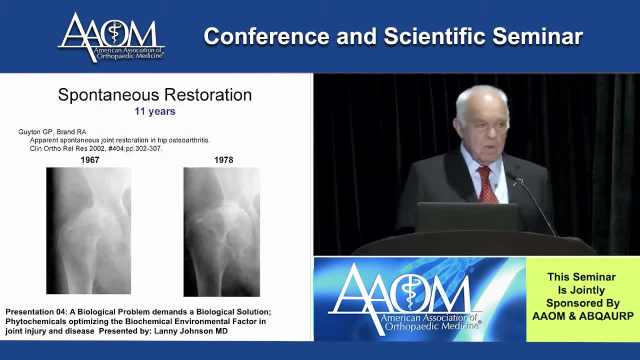 or the hip did this, But here's the one that really got my attention. Guyton and Brand from Iowa saw two patients came in, had a total hip on one side and were to come back in three months for the total hip on the other side. 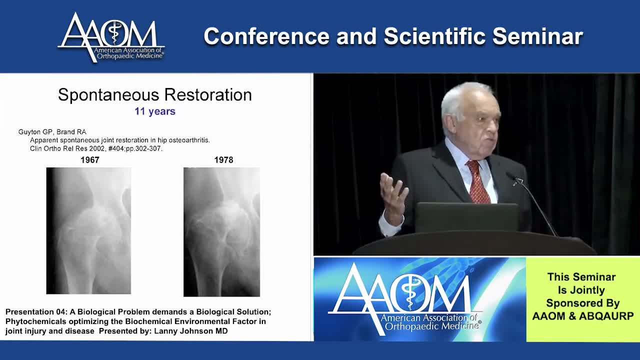 And when they came back in three months, they said: I don't want it, I feel just fine. And so they were not given any instruction on how to protect the hip, They weren't given any ambulatory aids, And they came back. 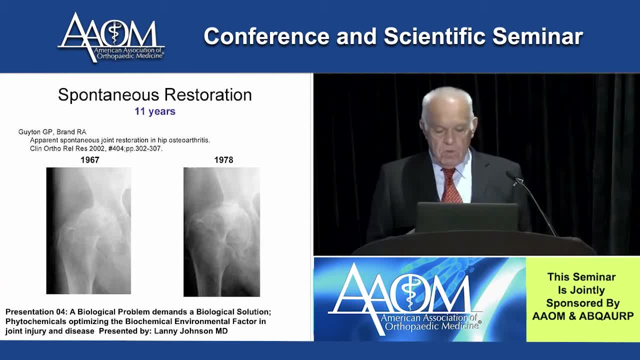 And so this first patient, 1967, that's when the doctor wanted to do the total hip. And finally, in 1978, they did the total hip. And there's what's happened, with no instruction. And how did the patient do this? 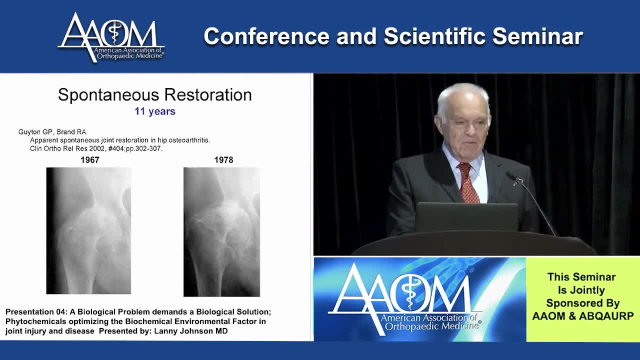 Well, they spontaneously unloaded this hip because they had a total hip on the other side. that didn't hurt. So every time they got out of a chair they did it with their total hip side protected. this. They always watched and did it that way. 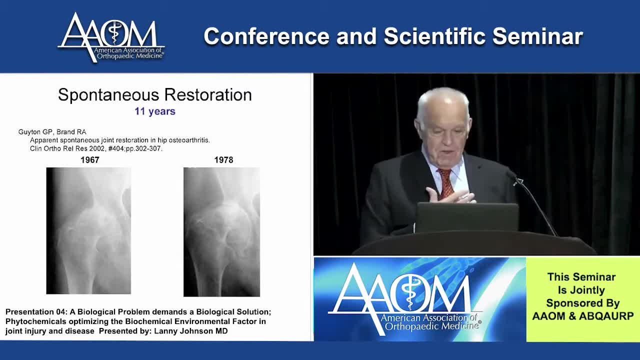 And so then, this one is even more amazing to me: 1994 to 2001.. No treatment on this patient, no instruction, no medication, no surgery, no stem cells, And the patient spontaneously unloaded from 1994 to 2001.. 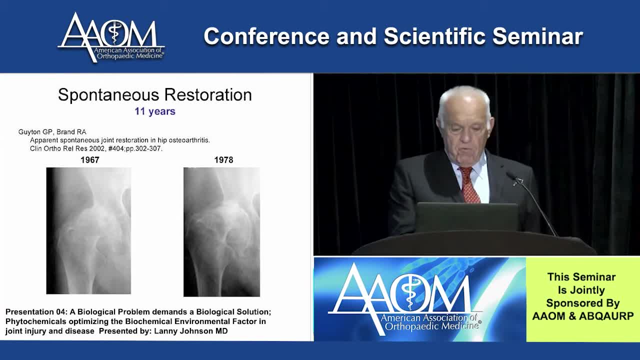 And look how. not only did their joint surface reform but also the bone remolded, which is absolutely astounding to me. But I think it's one of the greatest case-to-case reports that show the benefit of unloading, which is so often ignored in whatever treatments we're giving. 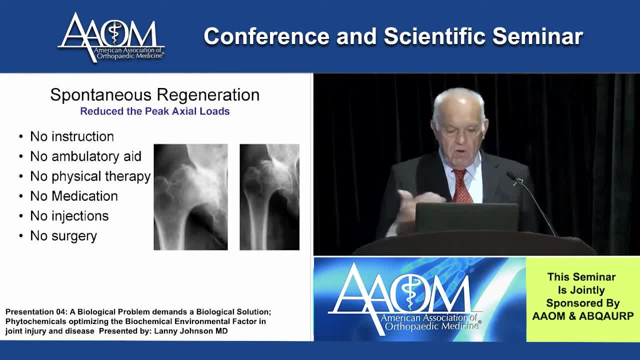 So here's these people: no instruction, no ambulatory aid, no physical therapy, no medication, no injections and no surgery. Now they subsequently had surgery. I don't know if the doctor just wanted the specimen or not. It's called Obamacare. 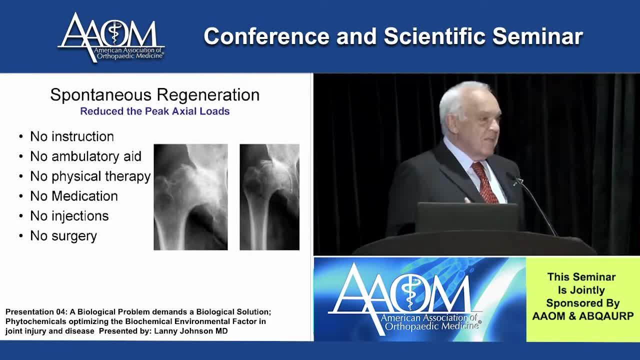 What There was, what It's called Obamacare, Yeah, okay. So what happened was that they were able to show the specimens and normal articular cartilage And you can look up their paper, because there isn't time to go through every detail. 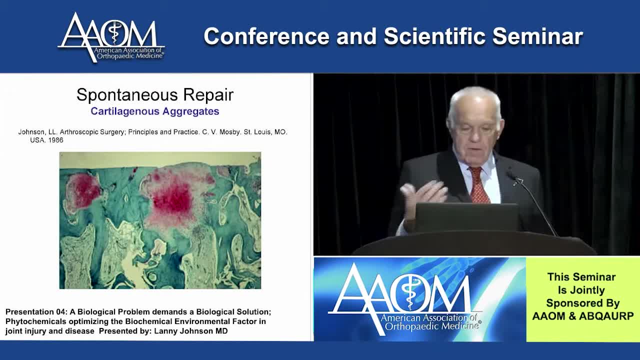 So why could this possibly happen? Well, in 86, in the textbook I wrote, I showed these cartilaginous aggregates on the surface. And so these cartilaginous aggregates have the opportunity to regrowth cartilage on the surface. 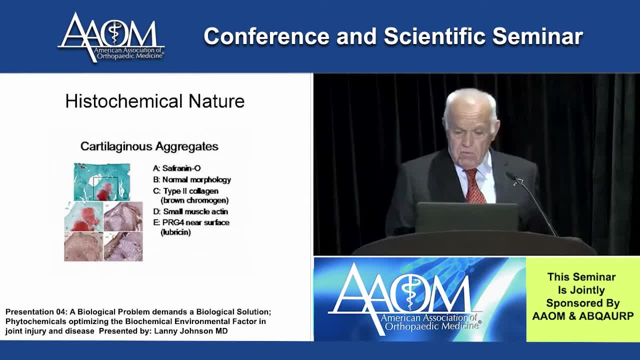 And we showed that they had in the substantive paper that they were positive. SAFO normal morphology had type II collagen, small muscle actinine, And so what we're seeing is basically an attempt on the normal natural history to heal this. 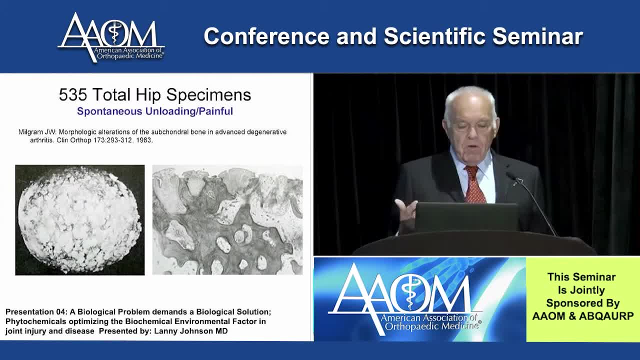 So what else was the evidence in the literature? Well, Milgram reported 535 total hip specimens, which were people who had a painful hip, so they obviously were kind of unloading it, And what he showed was that the surfaces were completely getting regenerated. 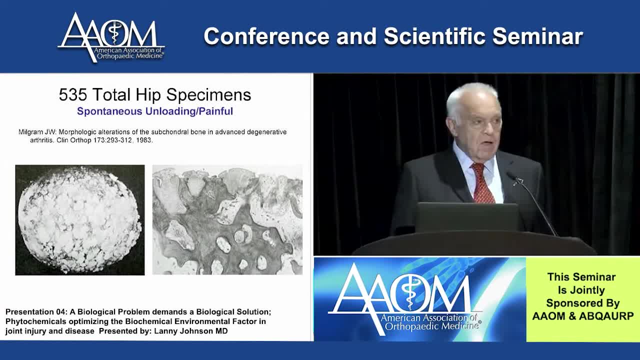 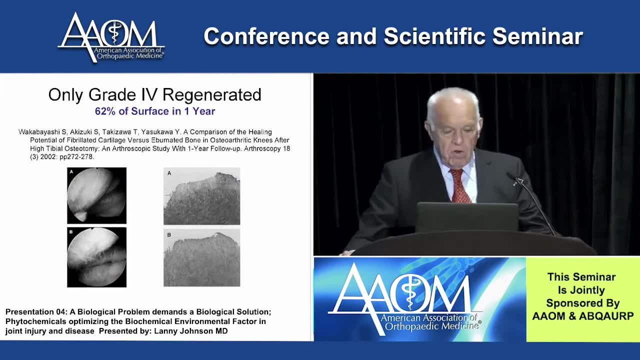 Even though they came to a total hip, they were completely regenerated by these cartilaginous aggregates coming up on the surface. So then there was a paper that even supported this more, and that was arthroscopically before and after high tibial osteotomy. 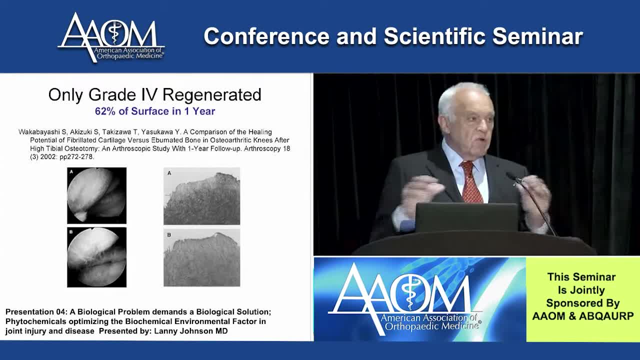 The one group had partial thickness lesions and the other group had bone on bone And only the ones that had bone on bone regenerated. The partial thickness lesions did not regenerate any cartilage to biopsy. So what we have to do here and the other aspect, 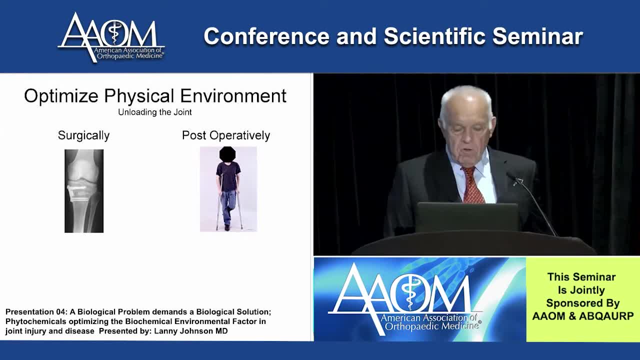 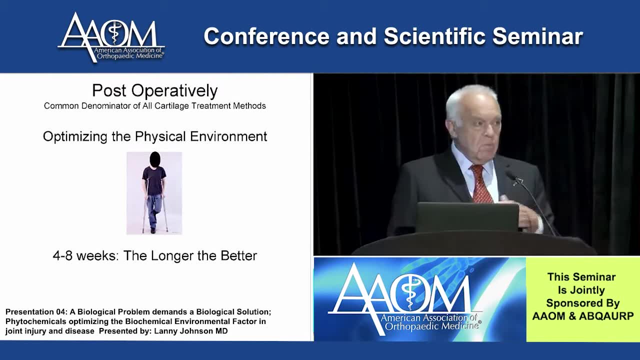 no matter what treatment you're giving, we've got to optimize the physical environment by unloading the joint post-operatively. So in my view, the common denominator of all cartilage treatment methods, even the non-treatment method, is the unloading of the joint, generally four to eight weeks. 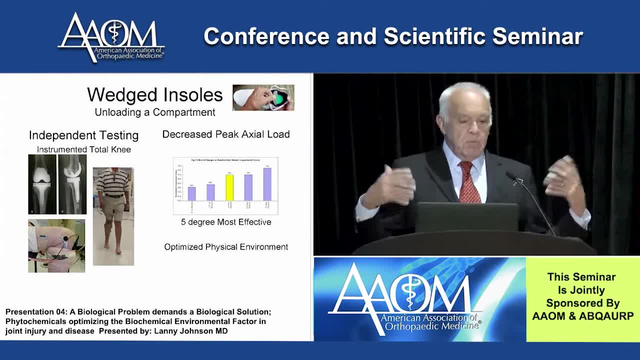 So then I took a look at what about wedged insoles. Could they possibly unload the joint? Very controversial in the literature, but at Scripps in California they had four patients who had an instrumented total knee that could measure the peak axial loads when a patient walked. 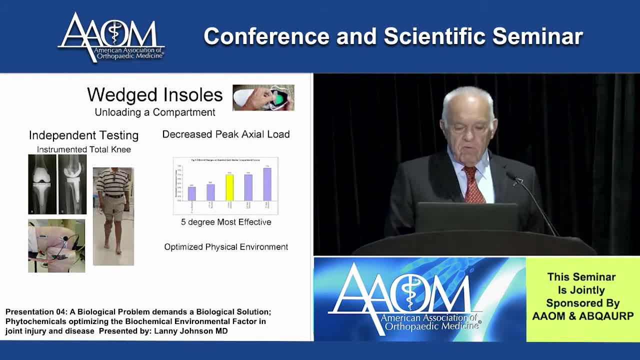 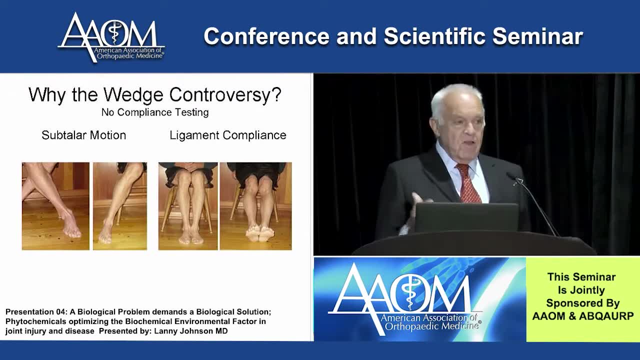 And we showed that with a five degree wedge insole that worked. Why is there controversy in the literature? Well, no one in the literature tumbled to the fact that you've got to have subtalar motion and you've got to have a compliant. 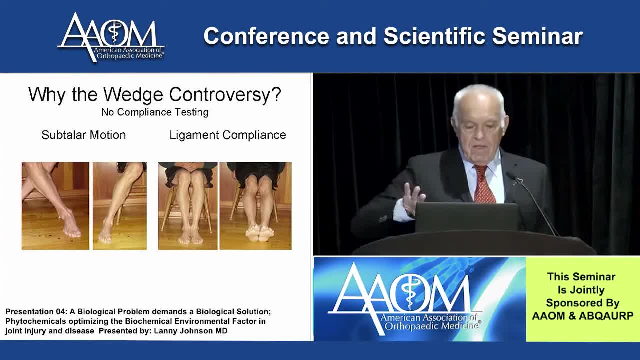 medial collateral ligament. Because if you can't have subtalar motion the way I showed here on the left side for either varus or valgus and you have to sit together and have your knees together, straighten them out, and if you can, hold your knees together, 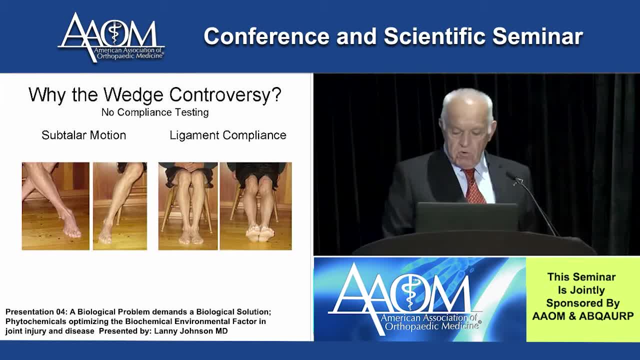 then the medial structures are compliant. No subtalar motion, no compliance. it wouldn't matter what the wedge did. A wedge cannot be powerful enough to overcome those structures. So there was a potential now, in my view, for either the non-operative treatment or, if you're going to have a meniscectomy. 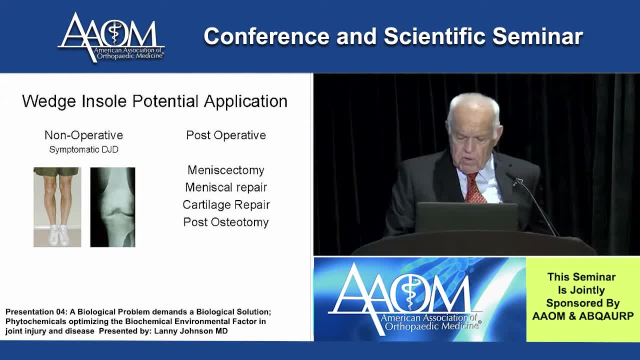 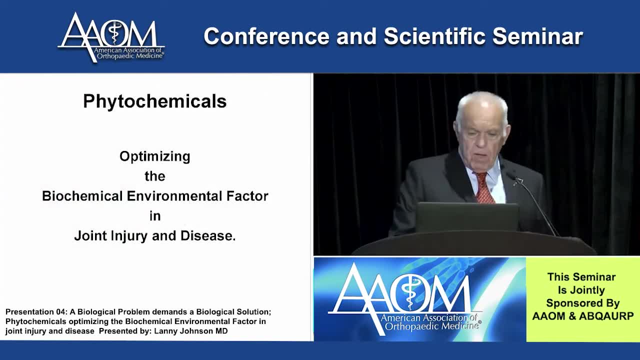 a meniscal repair, a cartilage repair or a post-osteotomy or any cell type treatment- that unloading the joint by this method would be optimal. Now let's take a look at phytochemicals. This is something I've been working on for about. 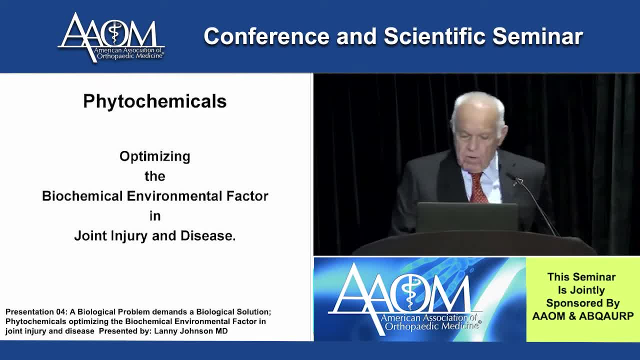 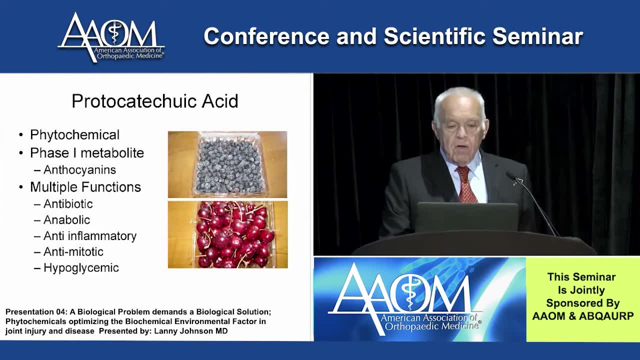 what more than 10 years And what it comes up with. we have a way to optimize the biochemical environment factor in joint injury and disease. Now what I'm going to talk about is a reagent called protocatoic acid. 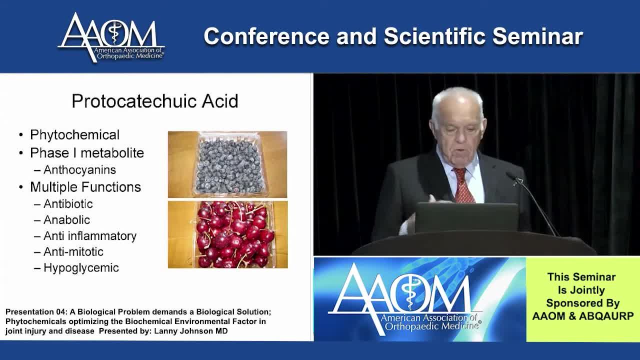 And it is a phase one metabolite that comes from what's known as anthocyanins- And anthocyanins are the dyes that are in blueberries, cherries and other plant material- And if you look this up, you'll see that it has a powerful antioxidant. 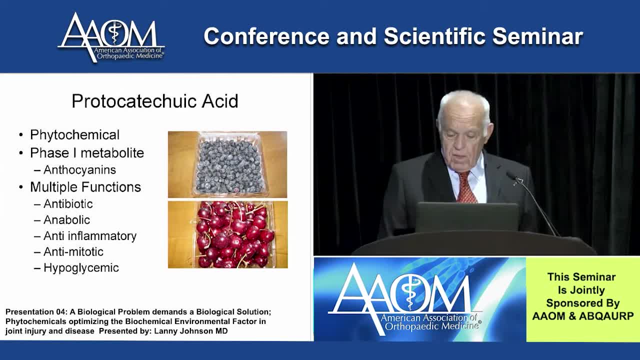 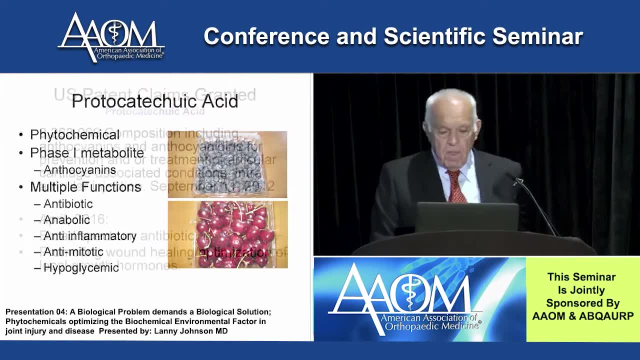 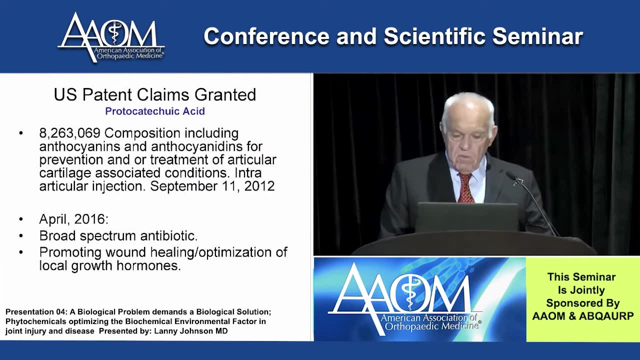 but it has antibiotic effect, anti-inflammatory, anti-mitotic and also can be hypoglycemic. Rather amazing what this does- And I was a granted patent in 2012, for the injection of these- how it would alter articular cartilage. 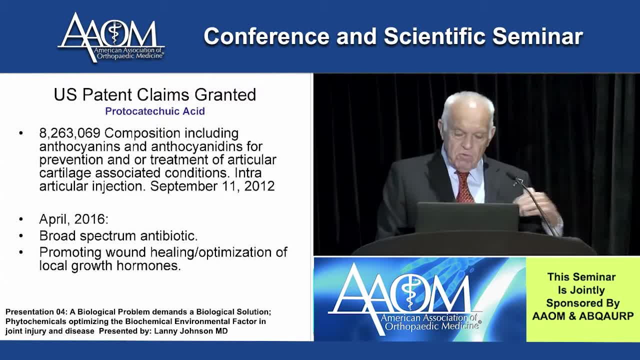 and affect the joint. And then recently I was granted another patent on the fact that it is also a broad-spectrum antibiotic in a different way, and that it also would promote wound healing by optimizing the local growth hormones. So now I want to turn 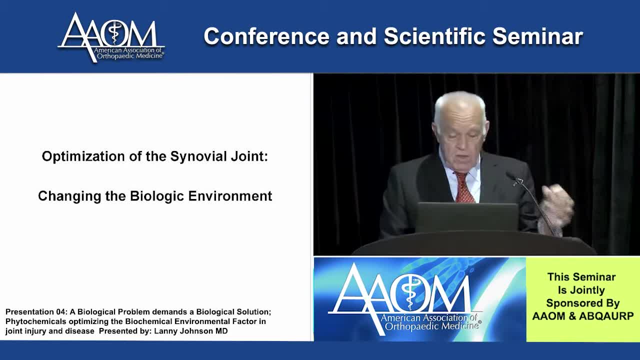 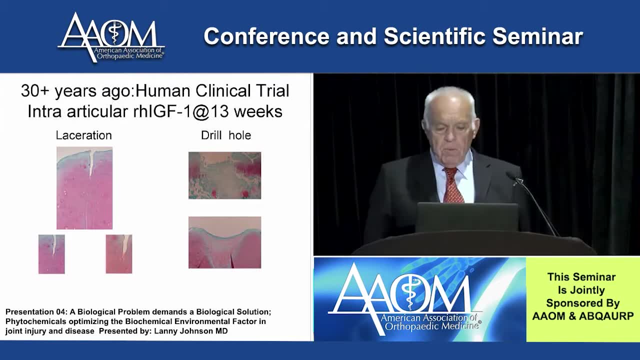 where I have a patent, and on the optimization of synovial fluid, that hasn't. I'm still waiting for my first patient, my first office action on that, And that started about 30 years ago when I was asked to help on a human trial. 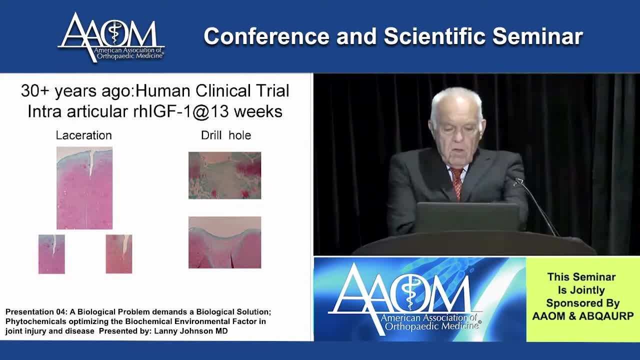 with a company called Chiron in Northern California and they used intraarticular recombinant IGF-1. And what we saw was there was sealing of the lacerations. These were humans who were going to have a total joint in 13 weeks. 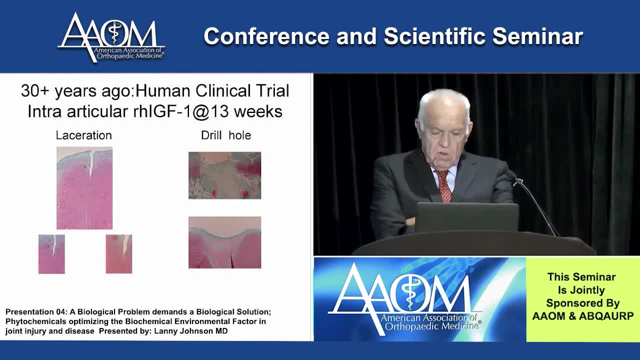 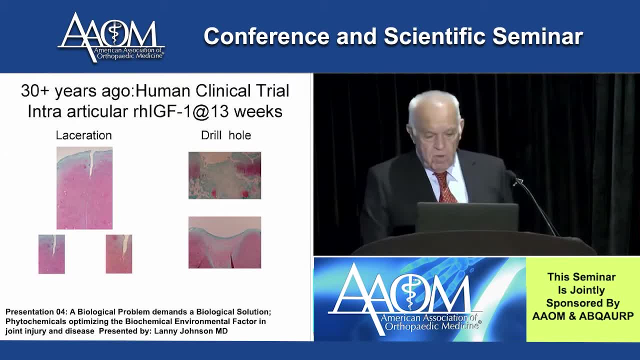 and we were able to go in arthroscopically, create the lesions and then get the histology And we saw that with IGF-1 in a human, which we already knew in animals, that it could have a beneficial healing effect. 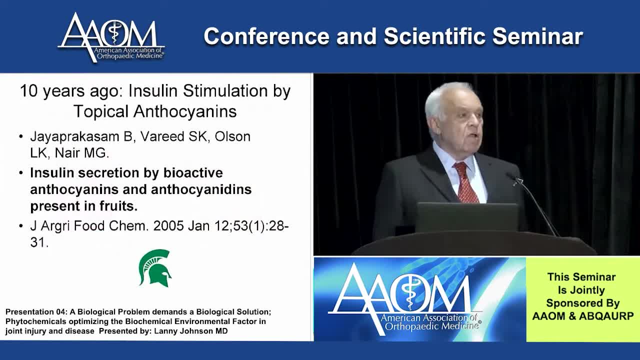 So that just kind of laid silent for me until about 10 years ago I saw that a lab in Michigan State University that they put insulin. they put the anthocyanins and anthocyanins on rat islet cells and it made insulin. 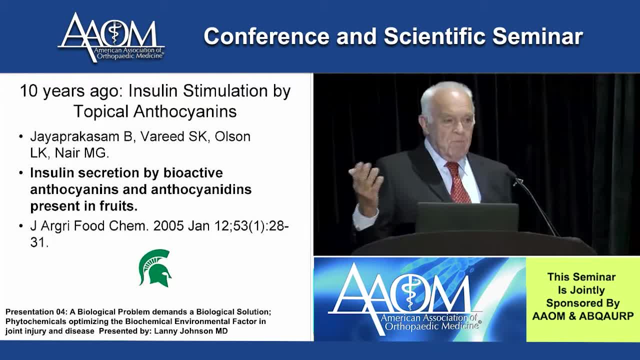 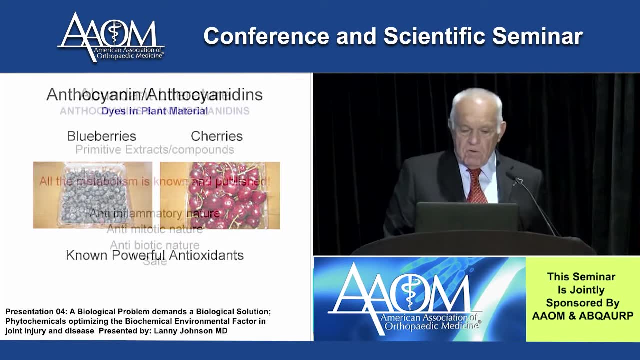 So then I raised the question: are there other places in the body where there are natural things that if we put anthocyanins on them, could we possibly have them make insulin? So that's when I went to think about going back. There are powerful antioxidants. 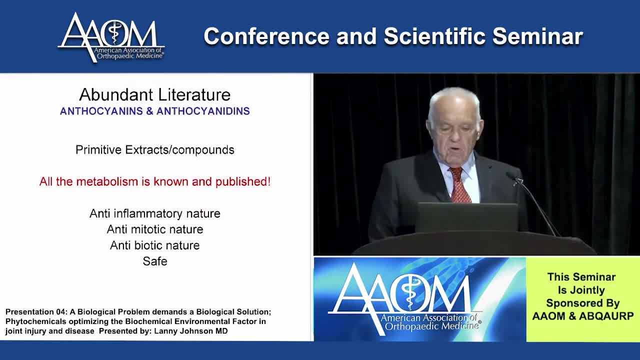 and let me give you a little background. There's abundant literature. Most of the work had been done with primitive extracts or compounds, and all of the metabolism is known and published: where it goes into your body, how it comes out of your body. 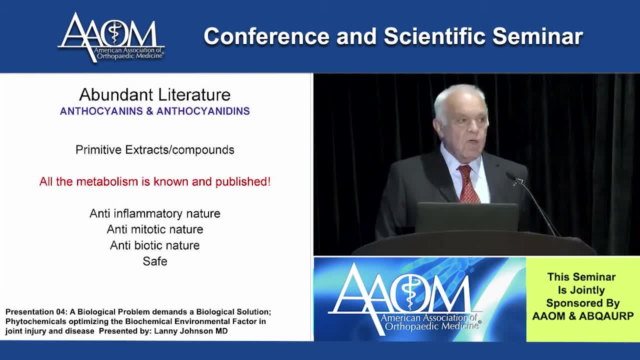 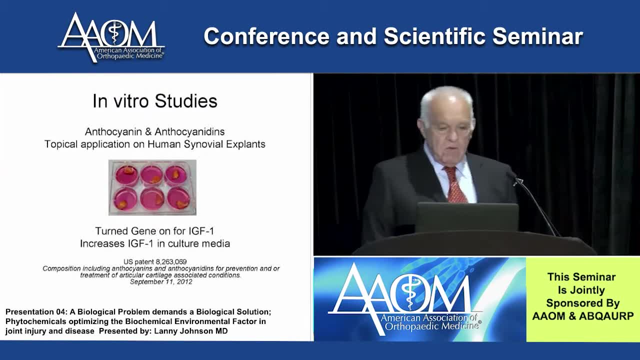 where it lands in your body and how long it stays there. So, unlike most drugs, if you're going to be worried about what's going to happen, the literature is filled with this. So then I went back to Scripps and I said: let's find out what can happen. 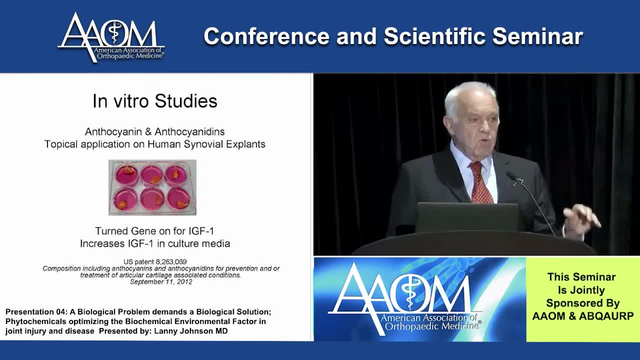 if we put it on human synovial explants that came from total joint patients And what we found out is it turned the gene on in the human synovium, or IGF-1, and increased the IGF-1 fluid in the culture medium. 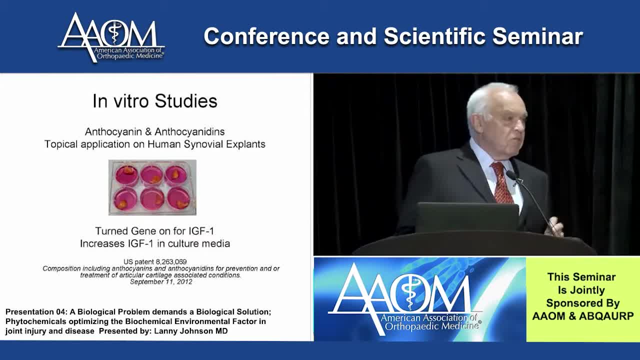 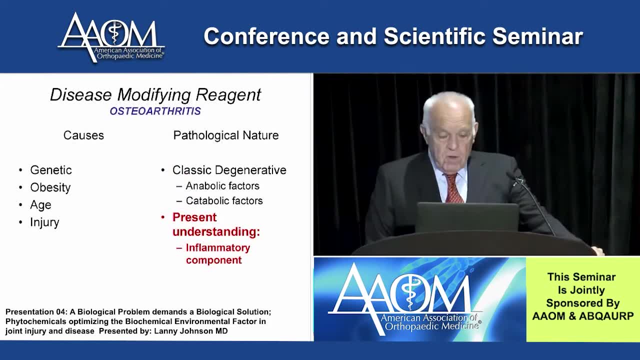 So it kind of supported my hypothesis there must be other tissues. well, there are more than just synovium, but that will benefit from this. So if we look at osteoarthritis, we have a number of causes and the pathological nature is. 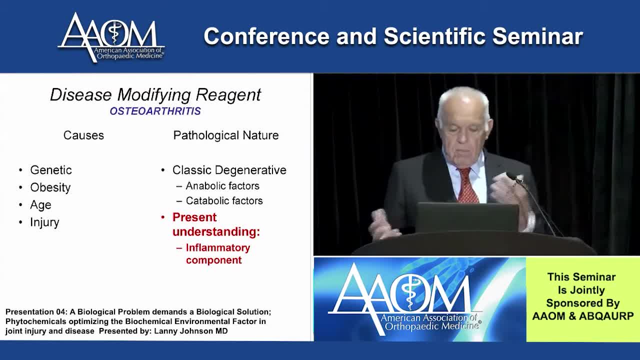 of course it's degenerative and there's a battle between the antibiotic and the catabolic factors, but one of the other present understandings is that it really has a major inflammatory component. So this: you have to know that the anthocyanins and anthocyanins 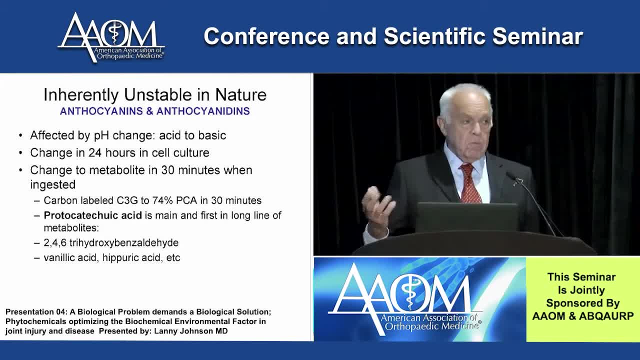 are affected by pH change. so if you put them in the human body, their acidic pH is 7, they very quickly metabolize, or also quickly metabolize in cell fluids, so that within 24 hours in cell culture it's protokyteric acid. 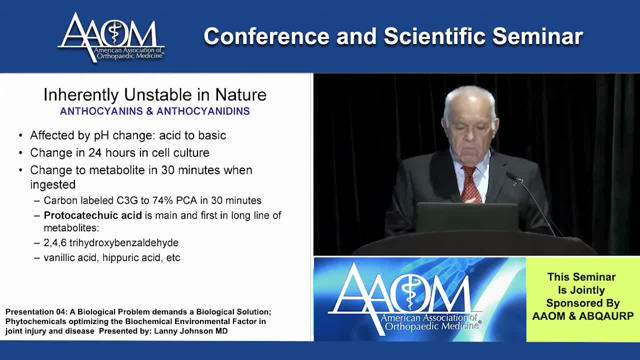 If you take it in your body by mouth, by the carbon label, they find out that every 74% is protokyteric acid in your bloodstream shortly after you take anthocyanins or these fruits. Now, you couldn't eat enough blueberries. 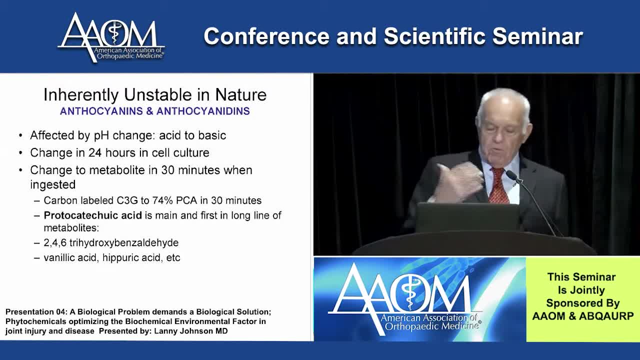 to get a dose of it. but if you take it in like 500 milligrams, you'll know that very rapidly it's in the bloodstream and then it goes down to phase one and phase two metabolites through your body. So what I started working with was 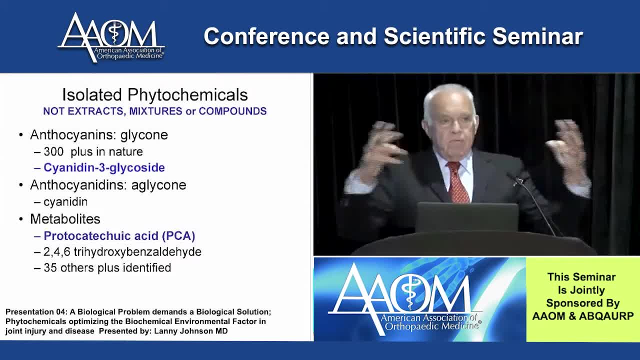 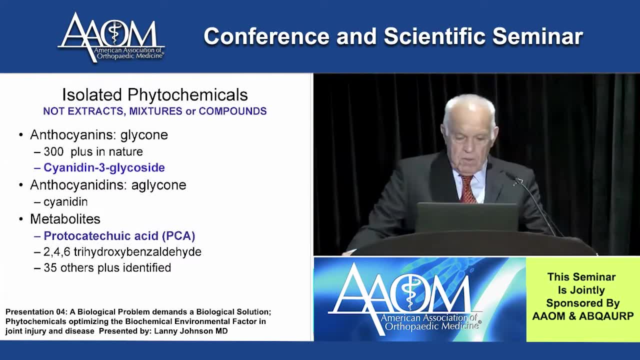 not extracts, where there'd be maybe 500 different things. you didn't know what they were. I isolated it down to cyanide and 3-glucoside, which was available and economically available, and also the main metabolite, protokyteric acid. 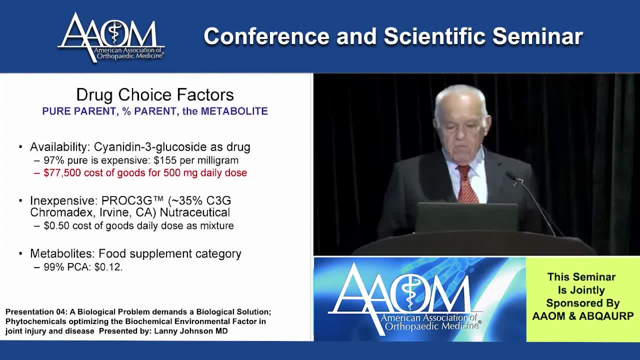 And so the problem with cyanide and 3-glucoside- that if you were going to give 500 milligrams a day it would only cost $77,500 a day to take the dose. so that was somewhat impractical. 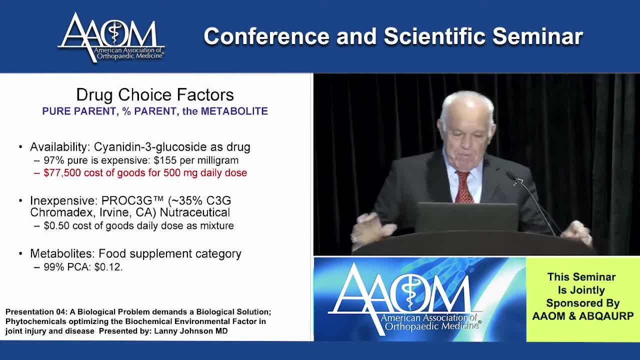 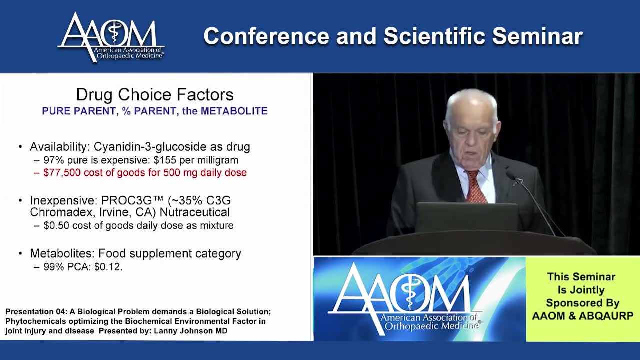 and even the government might support it, but impractical, expensive. So I worked with protokyteric acid in a 35% form and that would be about 50 cents, but down to 12 cents if we used the cost of goods for protokyteric acid. 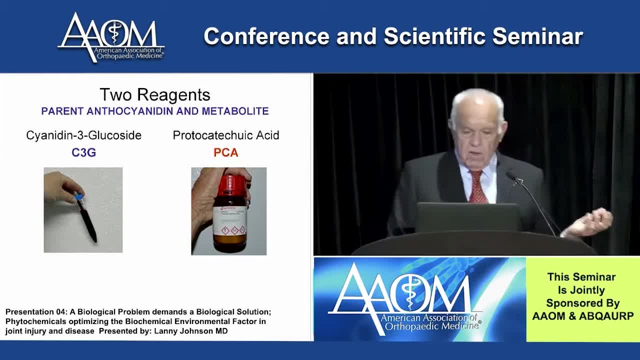 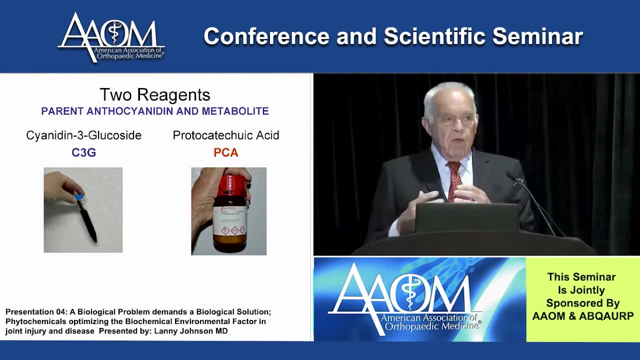 So then I did an animal study and I had done the injection and I showed that it happened. I could change the chemistry and I could have the synovium make IGF-1 by injection. but then it occurred to me: 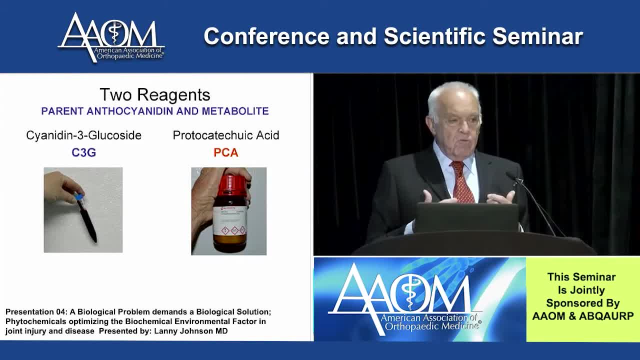 well, why wouldn't you take it by a pill? because if you can get it in the bloodstream, we're just as close to the blood vessels coming this way as we would by putting it on topically. And so then I did the rabbits this way. 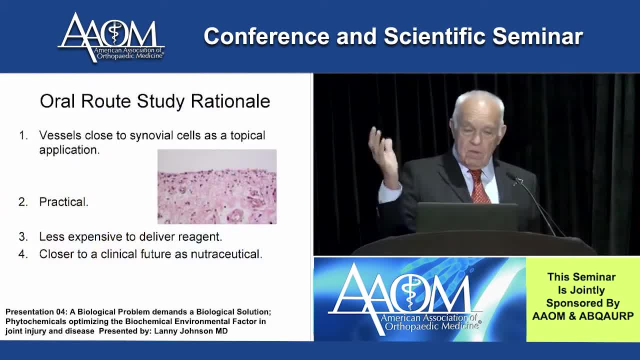 and I'll just report the oral ones. the ones by interarticular injection were the same. So with the vessels close to the surface, it was practical, less expensive and it was closer to a clinical future, because now it can be a nutraceutical. 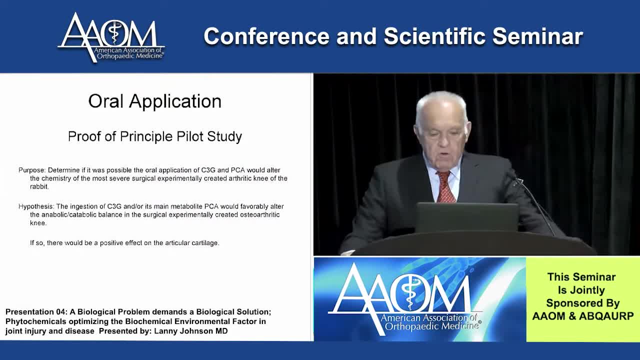 And so what we did was we thought that let's determine if taking Orale can change the chemistry of a surgically induced osteoarthritic joint, and my hypothesis was that it would favorably alter the anabolic-catabolic balance and maybe there'd be a positive effect. 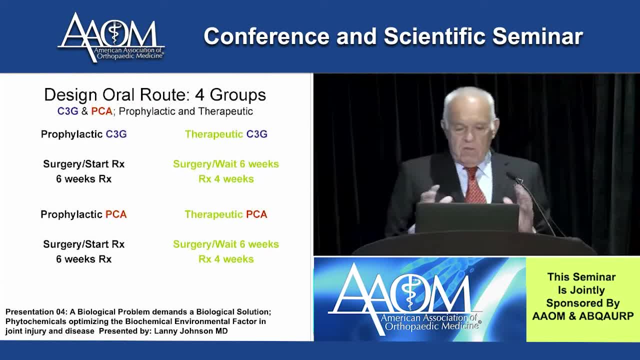 on articular cartilage. A little bit confusing on this slide maybe, but on the left is prophylactic in black and on the right therapeutic in the green. The prophylactics were started right away on the day of surgery. 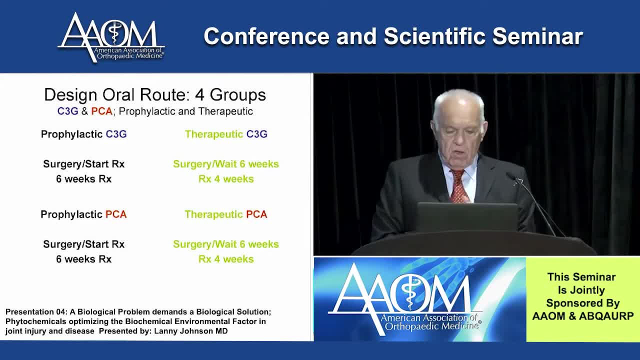 and I gave both reagents, cyanine-3-glucoside and protokytoic acid. On the right side, the therapeutic group, there were six in each group, bilateral knees on each side, and we waited six weeks and then had only four weeks of treatment. or took it out to ten weeks, And this is what we did. We severely disrupted the joint, cut the atypical collateral, took out the medium meniscus, cut the ACL and I was curious whether this would heal a laceration. 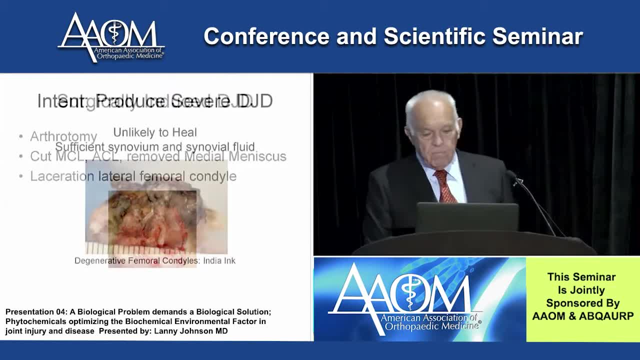 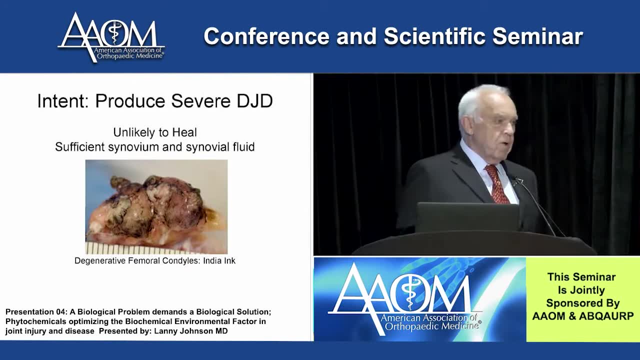 and so a laceration was made in the lateral femoral condyle. Now here's what those joints look like at necropsy. So I wanted to make sure you saw we were making the worst osteoarthritis you could possibly make. 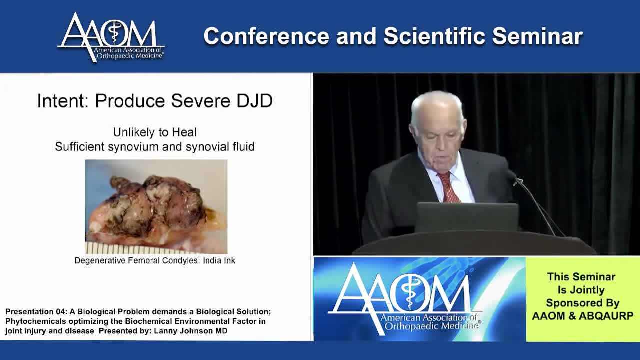 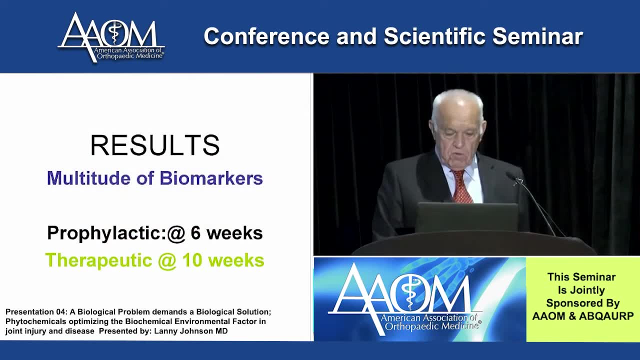 because I wanted to get the most synovial fluid I possibly could. So that part I accomplished. So we did a multitude of biomarkers. Remember, the prophylactics were six weeks, the therapeutic were ten weeks. So we first looked at inflammation. and on the prophylactic side, we saw that C-reactive protein was decreased by both, instead of being 8.8,. it was decreased with both reagents: the parent, cyanine-3-glucoside, and the metabolite. 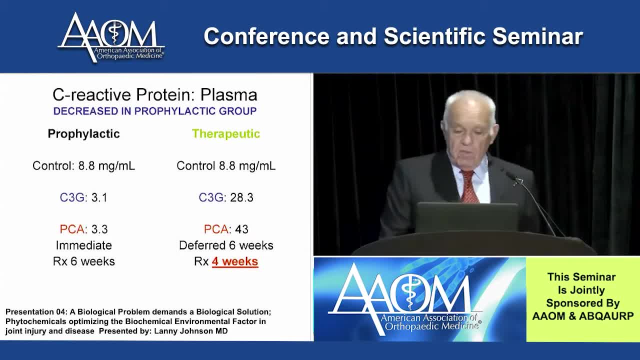 But the and not so on the preferred reason, and so that could have been. they only had it for four weeks as compared to six weeks, even though it was a delayed time. So I don't have the exact answer. I just know that it would work prophylactically. 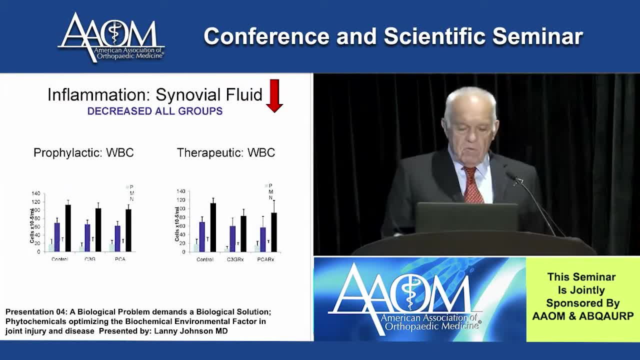 If we looked at inflammation and this. you can look at the slides on your own. I won't go over every one in the interest of a late afternoon time- but prophylactically we decreased the white blood count in all groups. 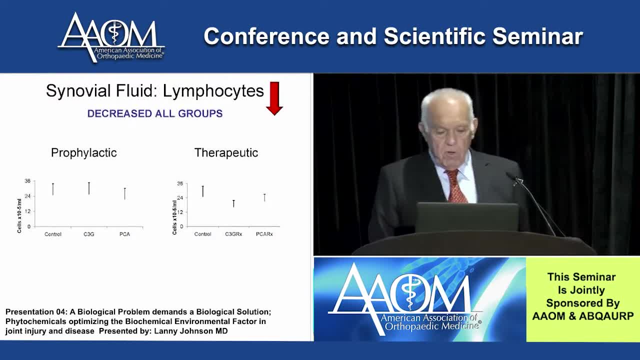 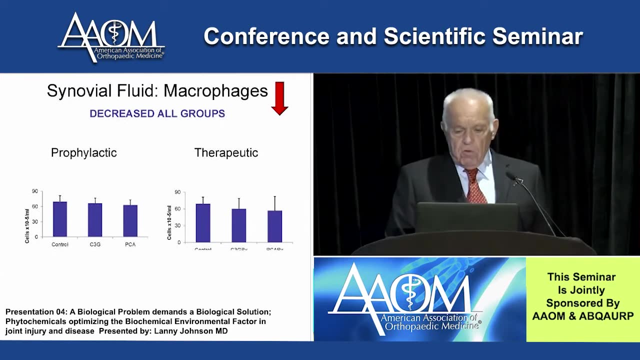 In therapeutic the same thing happened, And we also in both groups decreased the lymphocytes in both groups, both therapeutic and prophylactic, and for both reagents. And then the macrophages were decreased very slightly in all groups. 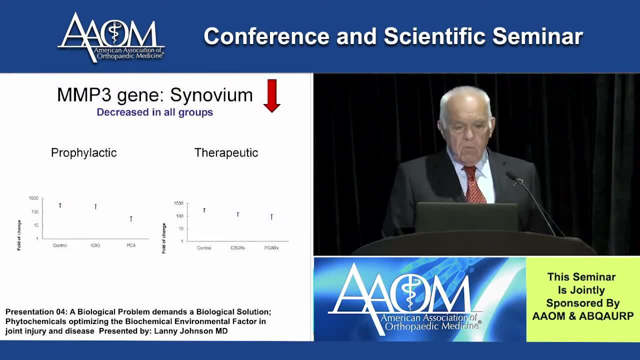 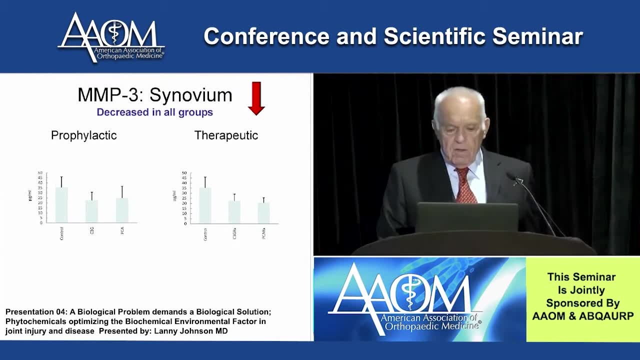 And the MMP3 gene in the synovium was decreased And the MMP3 in the synovium was decreased. So not only the gene but the amount And the lubricin was increased in the synovium And the in the synovium, the IL-6 cytokine, 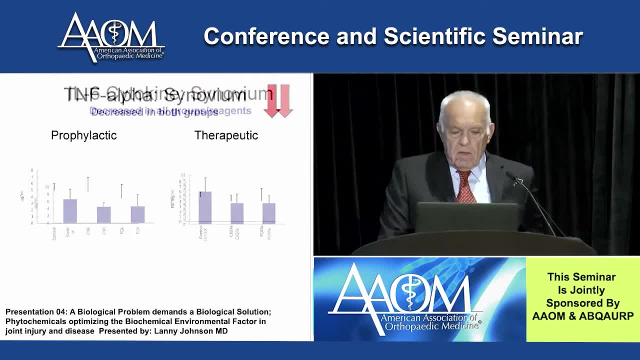 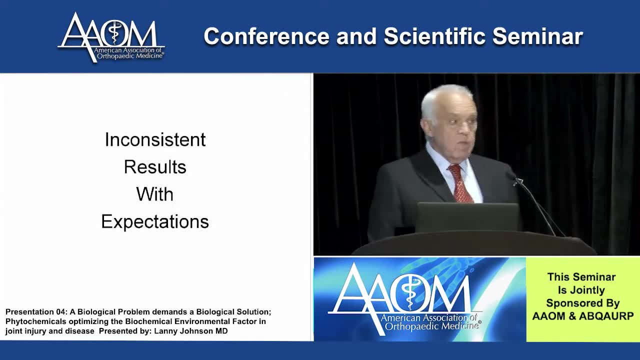 was decreased in all groups And the TNF-alpha was decreased in all groups, both prophylactic, therapeutic and for both reagents. But I had a lot of. everything wasn't perfect. I had a lot of inconsistent results that were with my expectations. 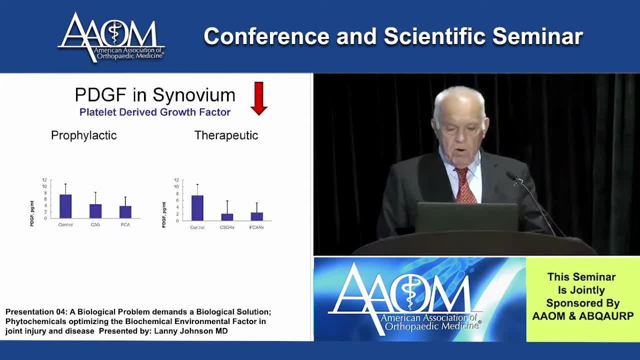 or one that weren't absolutely consistent across the board. So platelet-derived growth factor was decreased in all groups And TIMP1 in the synovium. the synovium was up and down and not consistent. It had a mixed effect. 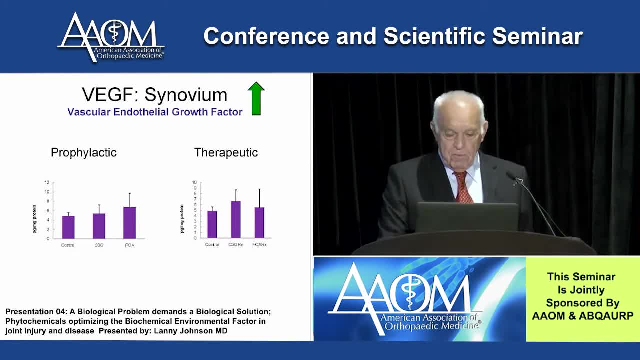 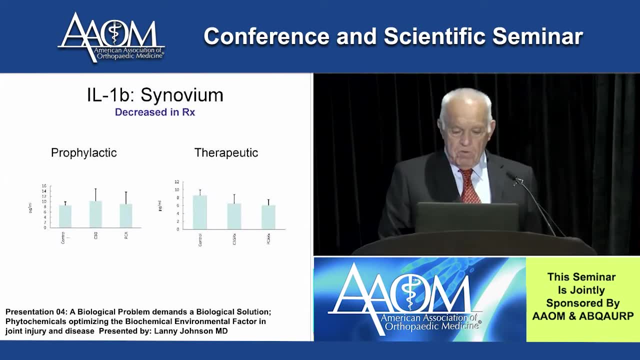 And BEGF in the synovium was increased. I thought it should have been. if I was predicting I would think it would be lower. And the synovium IL-1B was up in some and down in others, Not consistent. 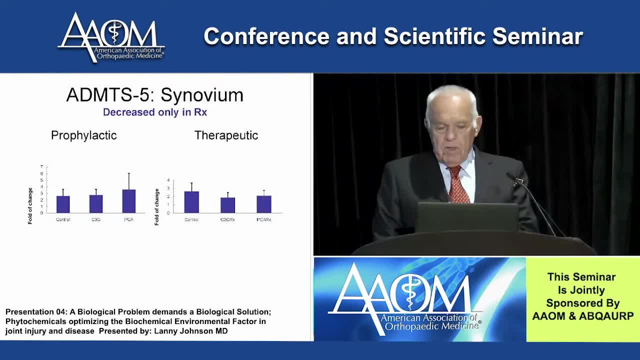 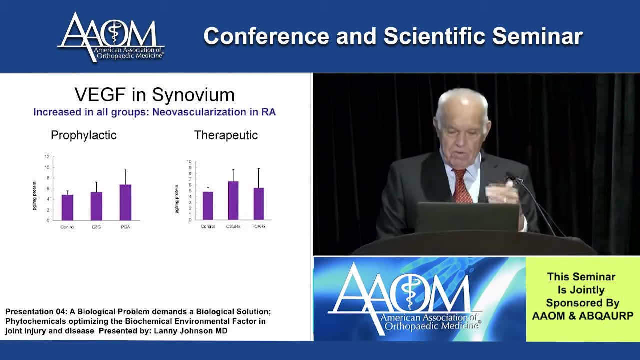 And 5 in the synovium was up in some and down, So again only decreased in the therapeutic. So I was learning that just everything isn't perfect. and the rest I I'll carefully go through now. What about? here's the bottom line. 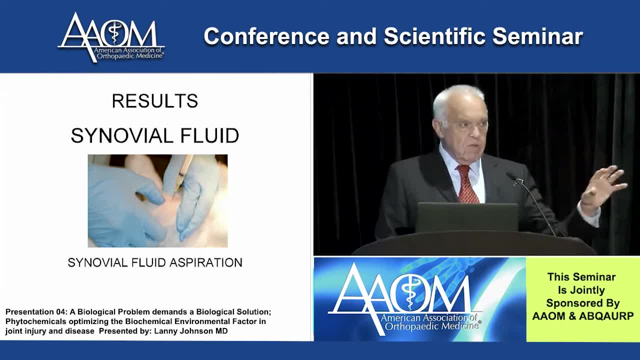 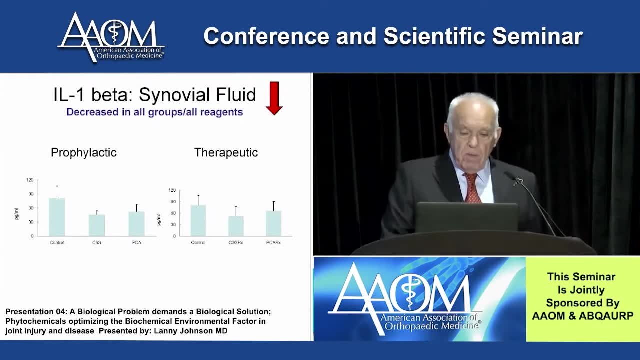 What about the results in the synovial fluid? I just talked about the synovium, how it was altered, Had the positive results that I decreased IL. it decreased IL-1 beta in both reagents and in both groups. MMP1 in synovial fluid was decreased in both groups. 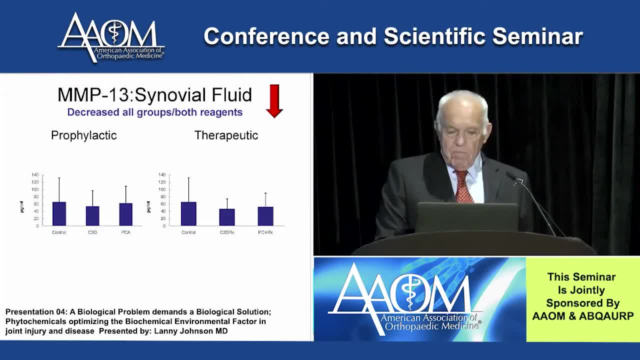 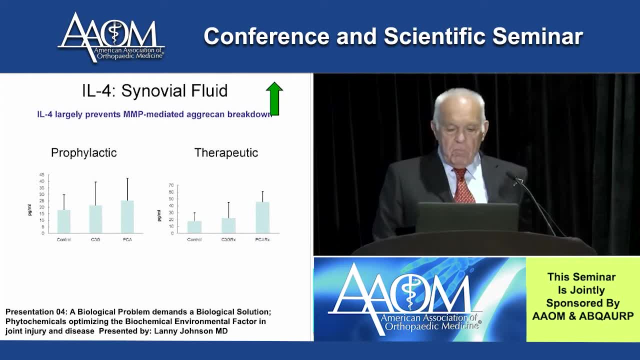 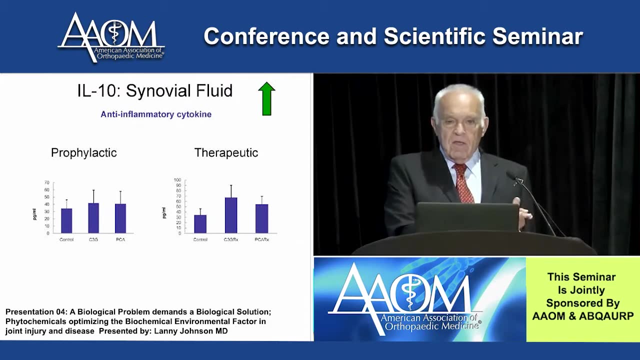 MMP13 decreased in all groups And then the beneficial cytokine, IL-4, was increased Compared to the control in both groups, And the same thing for IL-10. So I was having seen that I was decreasing the negative cytokines and increasing the anabolic cytokines. 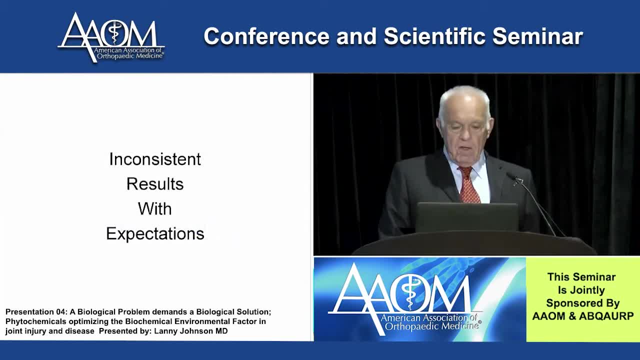 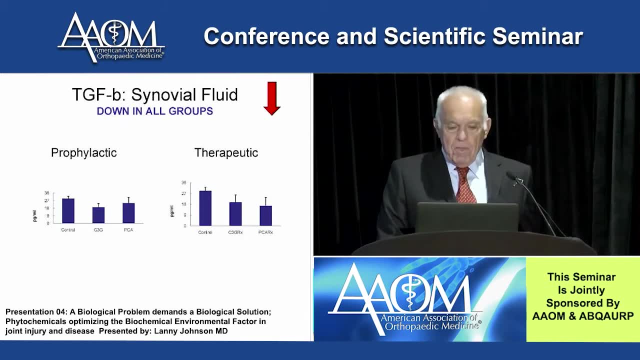 with this oral medication, Again, I had inconsistent results, which I won't take time to try to analyze every one. So some were down, some were up in the synovial fluid And in the interest of time I will go to the cartilage. 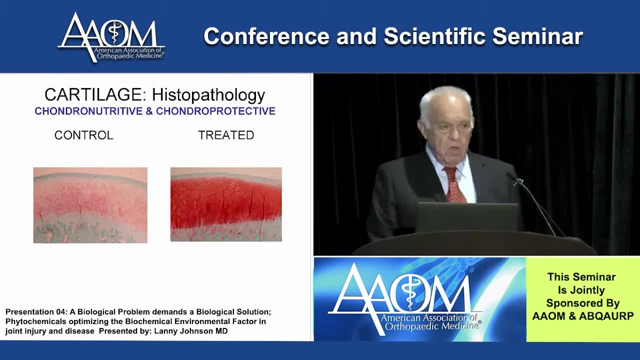 That's just the bottom line. So in the cartilage we found out that it was both chondro-nutritive and chondro-protective to the cartilage. So you see the control on the left with the SAFO and you see a treated SAFO on the right. 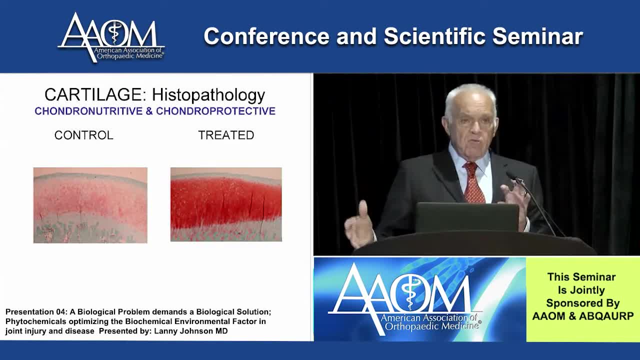 Now the lesion member was the medial compartment. I did a laceration of the lateral compartment. These are specimens from the patella which there wasn't any direct disruption except during the arthrotomy, And so what we saw with international cartilage. 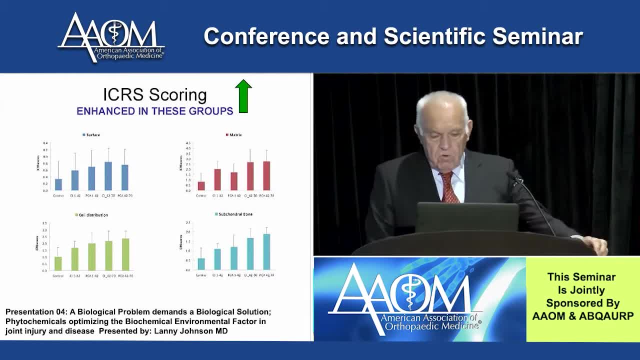 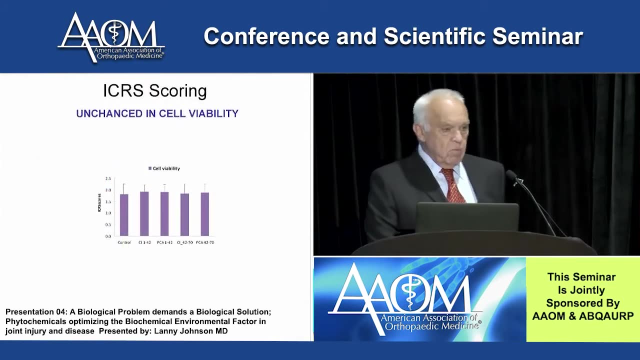 Research Society scoring. all groups were enhanced, So the surface was enhanced, the matrix was enhanced, the cell distribution was enhanced and the subchondral bone was enhanced. in all groups There was unchanged in cell viability, meaning there wasn't any degradation of it. 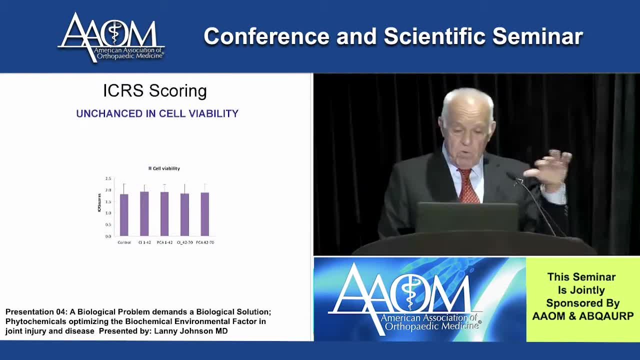 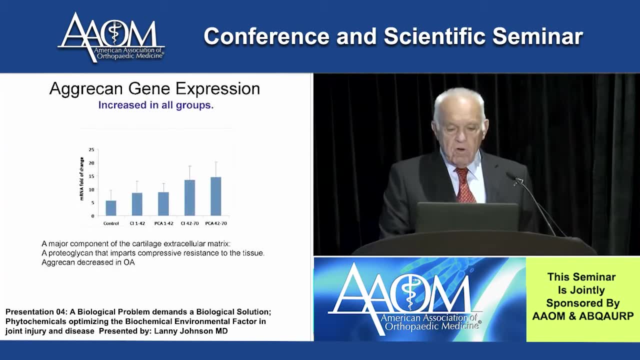 or any major increase, Because remember it stayed pretty normal. And then immunohistochemical scoring: we saw that the there was increased gene expression in the articular cartilage in all treatment groups, with both reagents And Lubricin was by the same method. 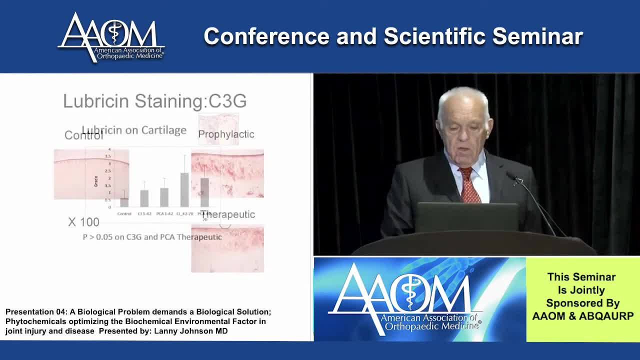 was shown increased in all groups. Here you can see a control versus the prophylactic and therapeutic, showing both increased staining of the Lubricin with the Cyanin-3-Glucoside and you see the increased staining of the Lubricin. 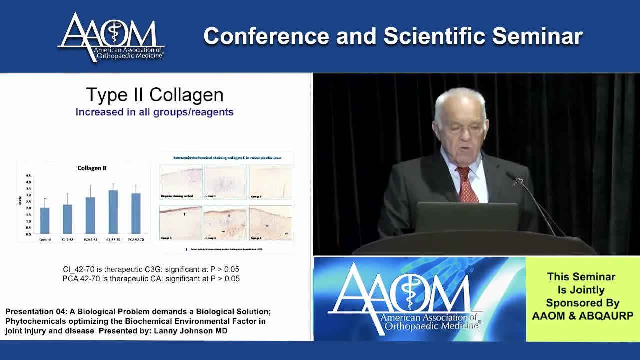 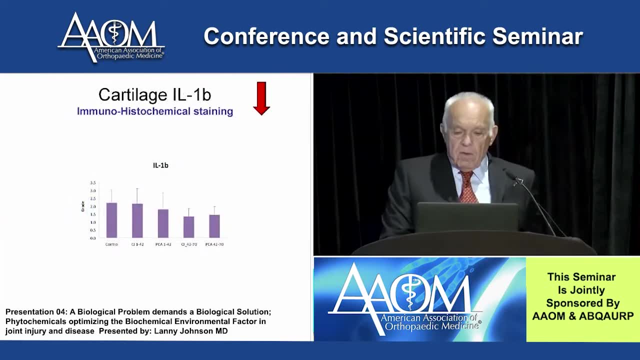 with the protocatoic acid And the type II collagen was increased as compared to the controls in all groups, all treatment groups, And then the in the cartilage, the IL-1B was decreased, especially in the therapeutic groups. 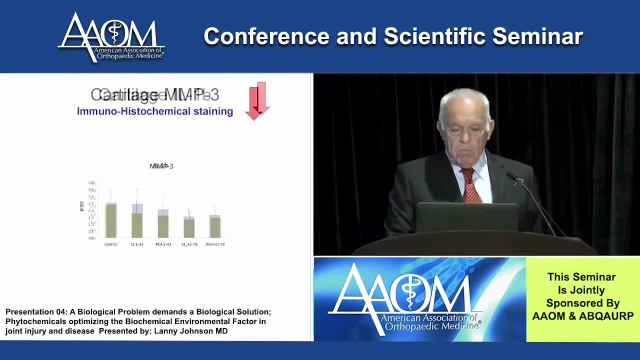 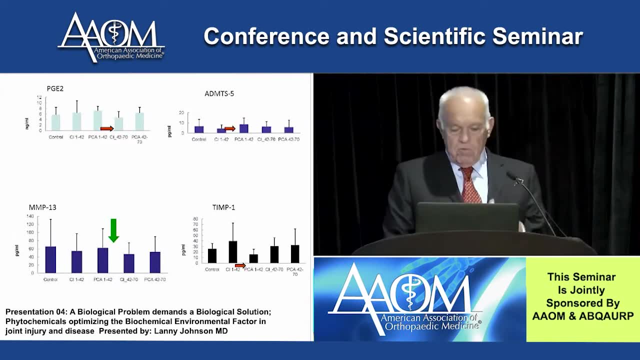 over to the right in both reagents And the MMP-3 was decreased in all groups in the cartilage. But again I had inconsistent results which some were up and some were down. Each would take a little bit more explanation than is necessary. 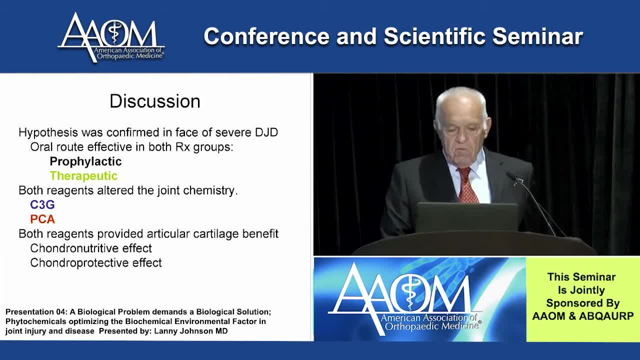 But a hypothesis was confirmed in the face of severe degenerative arthritis that the oral route was effective in both treatment groups, both prophylactic and therapeutic, and with both reagents, and that there was a chondro-nutritive effect and a chondro-protective effect. 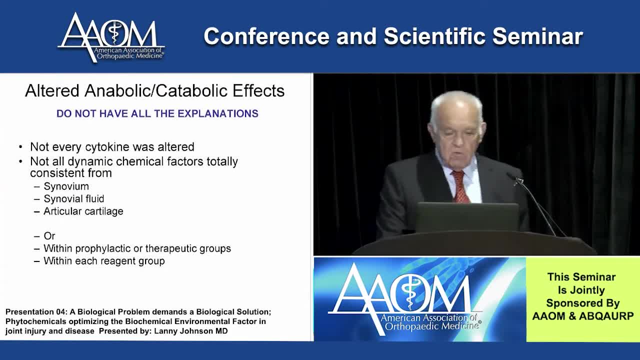 I did not grow cartilage. I don't have all the explanations. Not every cytokine was altered, Not all dynamic chemical factors were consistent across synovium, synovial fluid, articular cartilage, But there and it wasn't exactly the same. 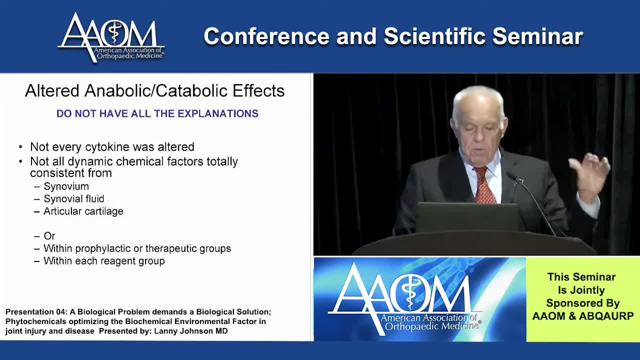 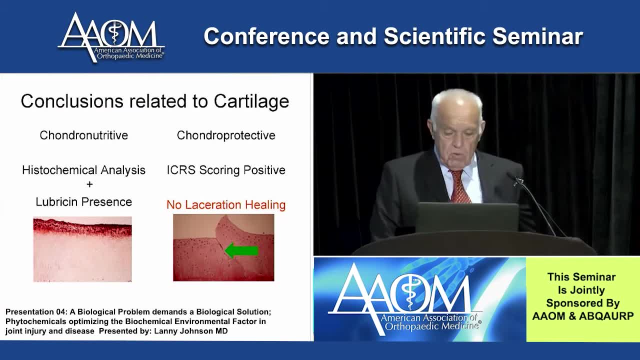 whether it was prophylactic or therapeutic, But in general we're able to make a major change in that chemistry Now. so it was chondro-nutritive, because what we saw especially happened to Luberson. But I did tell you I made a laceration. 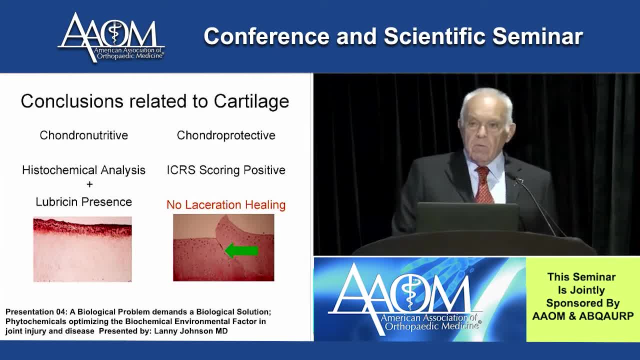 on the lateral side and there was no laceration healing. And there isn't laceration healing for a couple reasons. One: it will not house and hold a blood clot. Number two: it's moving all the time, So there isn't much of a chance. 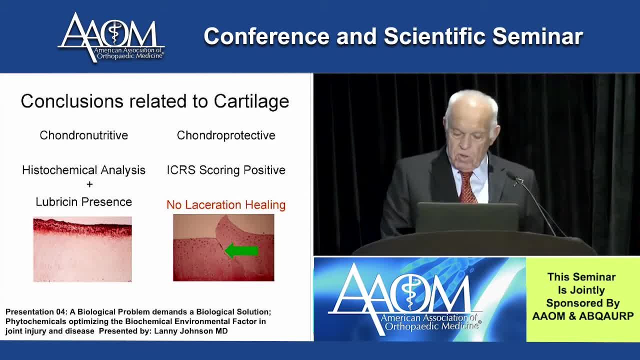 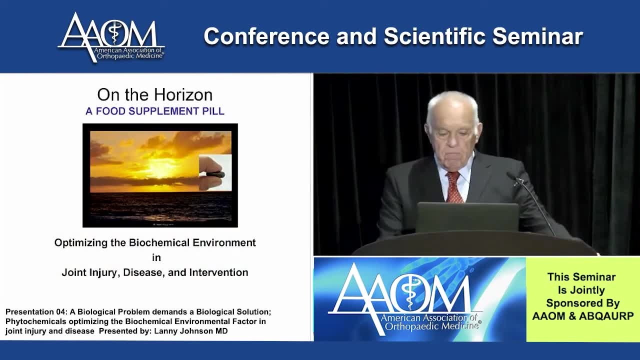 in a partial thickness laceration. If you drill a hole down in the bone then I know you can get a laceration to heal, but not a partial thickness one. So on the horizon, I believe there's a food supplement pill. 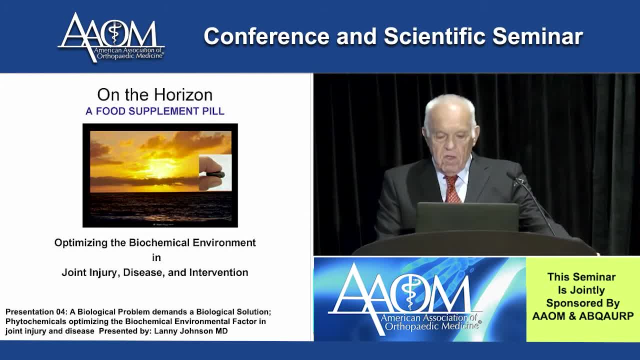 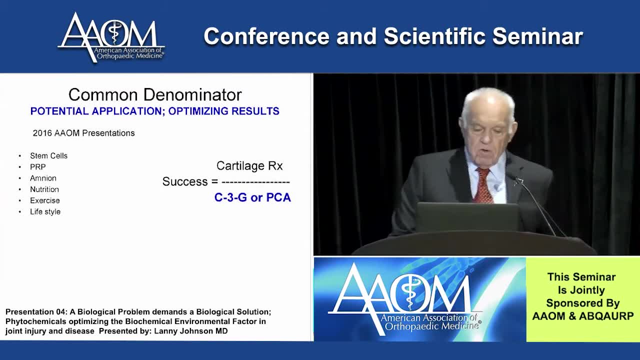 that will optimize biochemical environment and joint injury, disease and intervention. So, no matter what- and these are the presentations that were made at this meeting- stem cells, PRP, amnion, nutrition, exercise or lifestyle that I believe one of the common 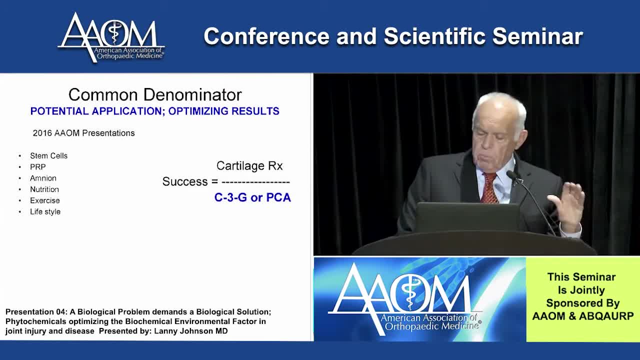 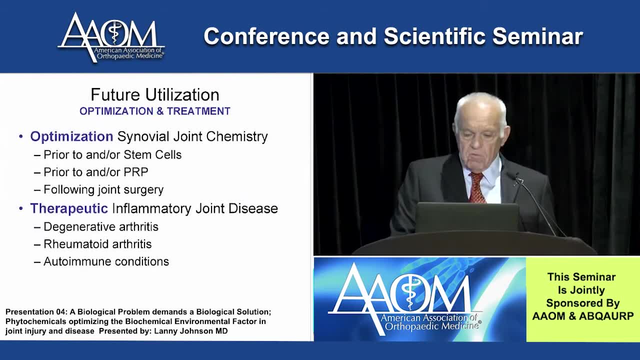 denominators for success will be that IGF, protocateteric acid, or cyanine and 3-glucoside, prophylactically before or after. So we can optimize the synovial joint chemistry and there can be a therapeutic. 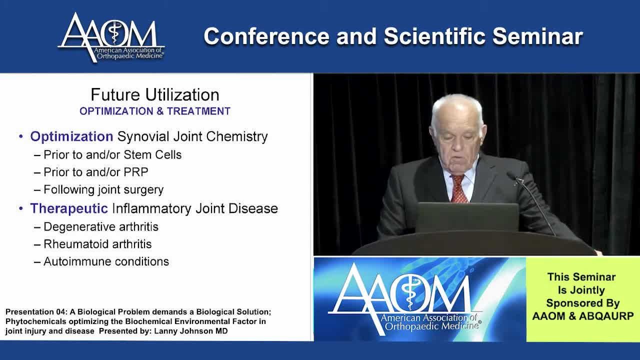 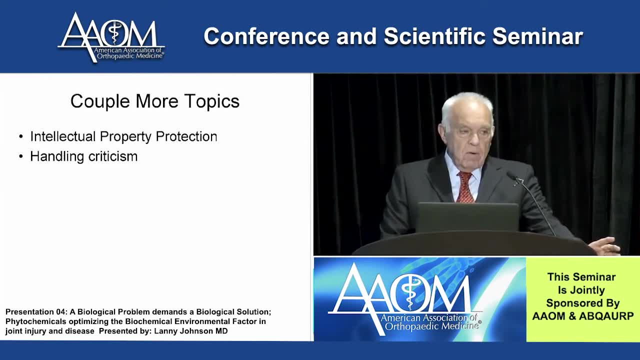 and inflammatory disease, no matter what it is, can be altered by this. Now, how are we on time? I'll go over a couple short topics, or I can stop. It doesn't matter, It won't even take five minutes. 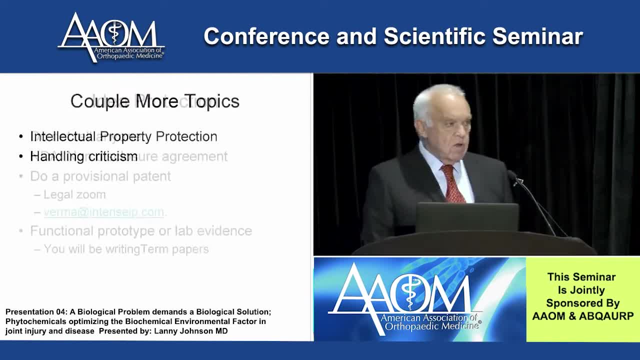 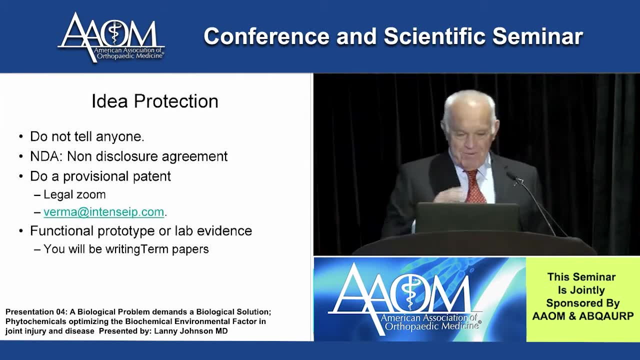 Okay, this is. a number of you might have an interest in intellectual property. So here's: I have over 60 US patents in medicine. I have 10 in golf. That's in the last few years. First of all, don't tell anyone your idea. 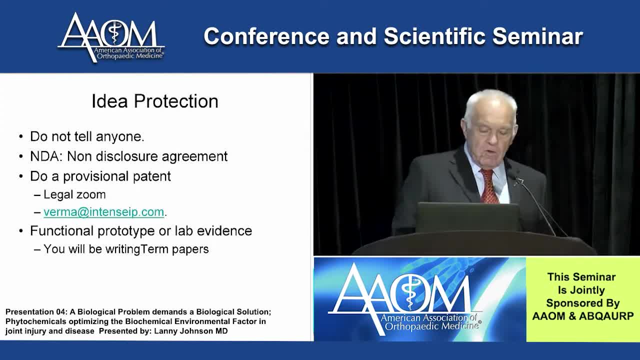 And if you're going to talk to somebody that's not a business, you might have a non-disclosure agreement, but you don't need an NDA if they're a business, and I'll tell you why in a minute. The next thing you do is you do a provisional patent. 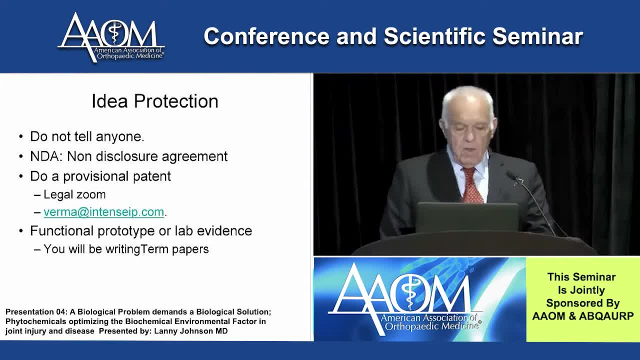 and you can do it inexpensively and this is written up in your handout at either LegalZoom or at this website. I've used from India and they do a nice job and relatively inexpensive. And then you want to make a functional prototype. 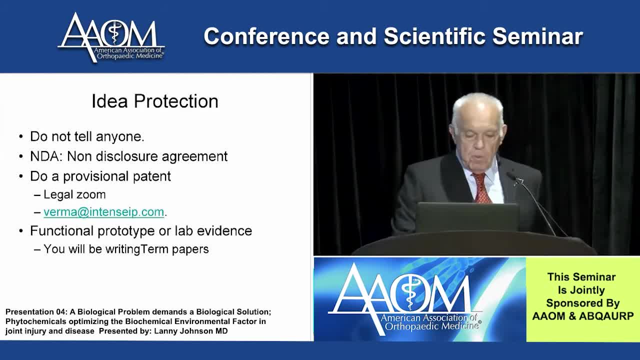 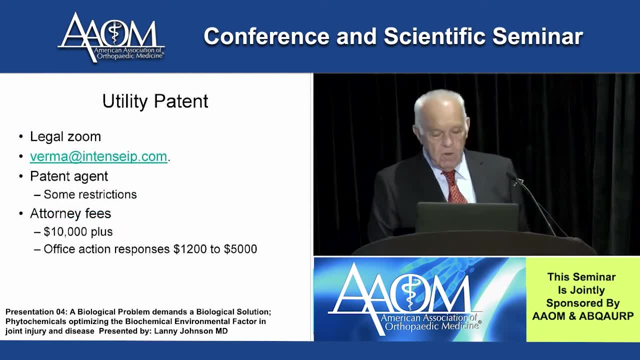 or have some lab evidence and you'll find yourself you'll be writing a lot of what I call writing term papers, because you'll just be doing literature, research and writing. Then you want to go to a utility patent If you still want to save money. 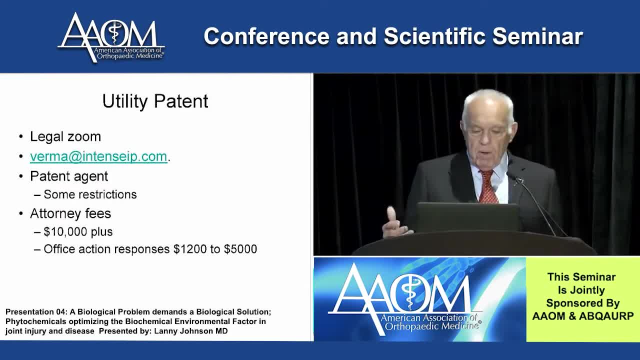 you can go to the two sources that I gave you, or you can go to a patent agent, but they have some restrictions and if the year you have from the provisional to the utility allows you to really find out if you've got something, whether you want to spend a lot of money or not, And so if you go to an attorney, you might get it done for $10,000, but if it's something chemical, you can look at $25,000 to $50,000. because of the office actions from the patent office. So they often cost between $1,200 to $5,000 each time they write you a letter and your lawyer responds. So you want to make sure you really got something before you carry it this far. 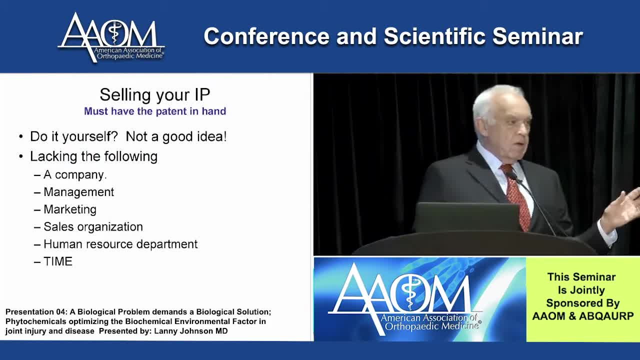 Now, what about selling your IP? First of all, you must have a patent in hand. If you don't have a patent, don't go talk to anybody. And there'd be two ways you could do this. One: you could say: 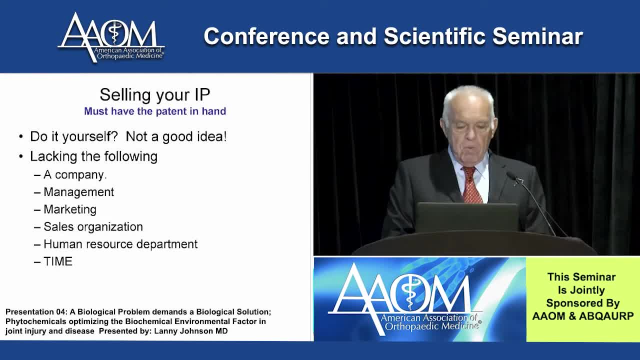 I'm going to not talk to anybody. I'm going to market this myself. I personally do not think it's a good idea because generally you will lack the following: You won't have a company, You won't have management, You won't have marketing. 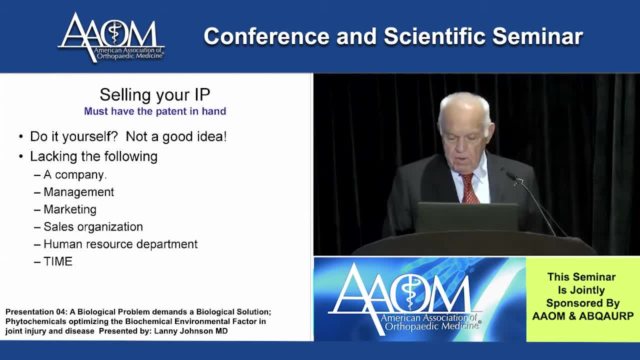 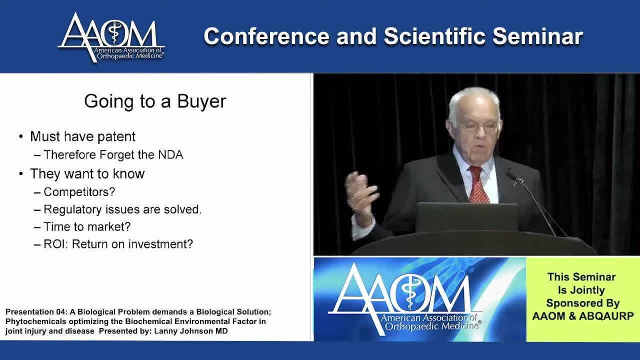 You will not have a sales organization, You'll not have a human resource department and you probably won't have time. So I'd recommend, if you have a patent in hand, find somebody who will buy it. Now remember if you're going to a buyer. 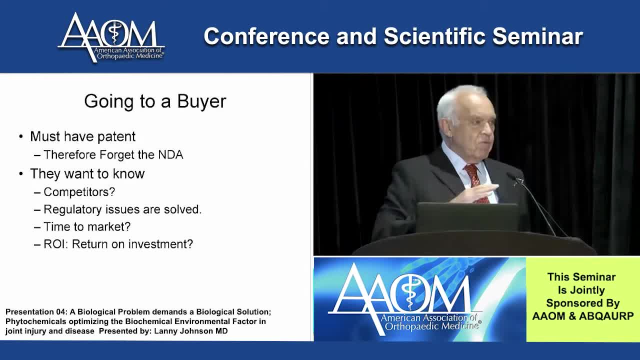 you must have a patent. Therefore, forget the NDA. If you want to have a patent, forget the NDA. Now here's what they want to know: Do you have any competitors? Have you got all the regulatory issues solved? 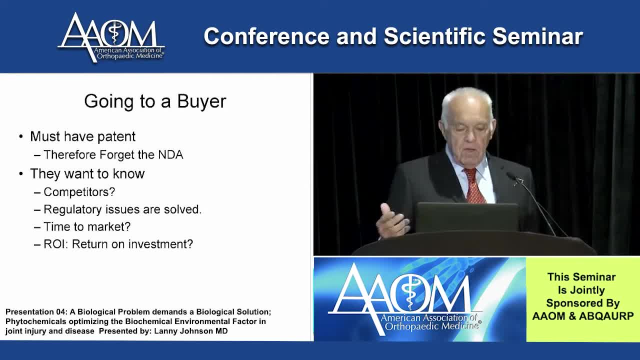 Of course, the answer's going to be no, because you've probably already done that. How long will it take to market this? And then, what they're mainly interested in is not medicine. You need to know that. They're interested in money. 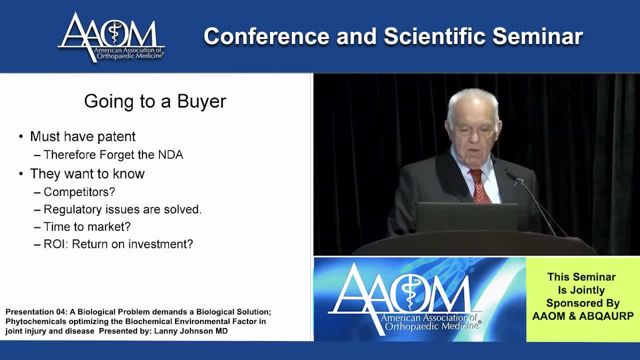 And so they want to know what's the return going to be on that, What's the return going to be on their investment? And here's the mind of the buyer, And you should know this: They're not a buyer, They're a robber. 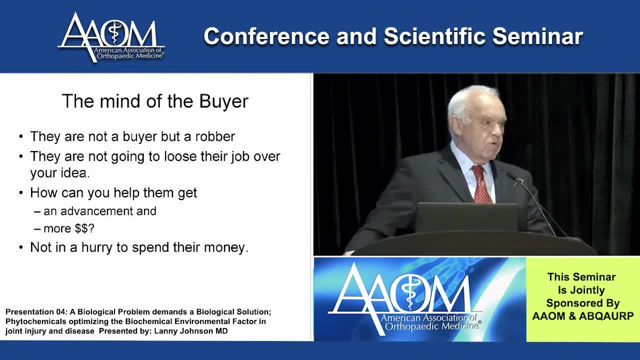 And so they're generally going to try to find out how they can get this from you for free or for very little. And the other thing is, when you meet one of the junior men at the company, they're going to say- and I say this: 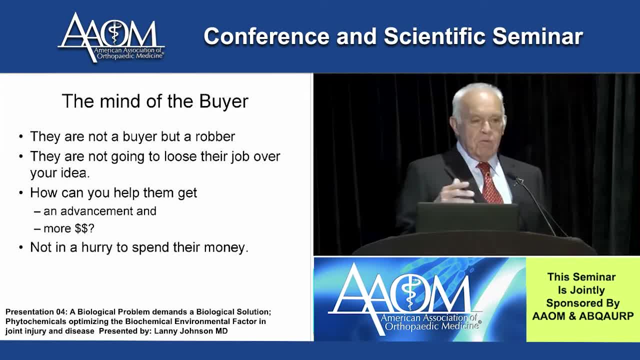 I even tell them up front: I have this idea and I want you to know. I know you're dealing with the fact you don't want to lose your job over Lanny's idea, So they don't want to get into this too far. 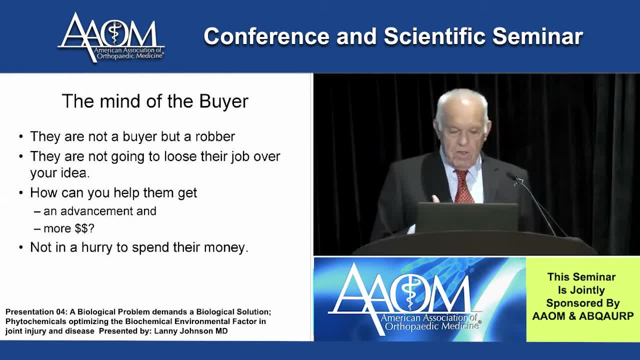 because they're interested how you can help them. Can you give them an advancement? Can you get it so they earn more money in their job And they're also not in a hurry to spend their money? Now let's take a look at the battlefield of change. 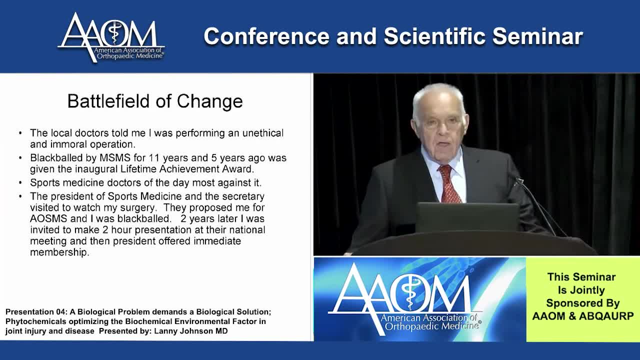 that you're facing And I will briefly tell you that when I started arthroscopy, the doctors in my town were nice enough to come and tell me that I was performing an immoral and unethical operation. doing arthroscopy- Now we know it's the most common. 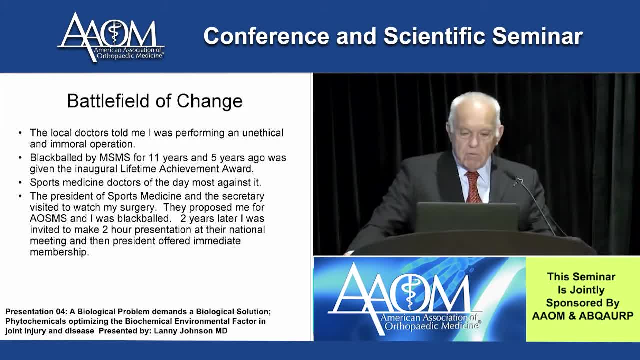 immoral and unethical operation. I was blackballed by the Michigan State Medical Society for 11 years, and five years ago I was given the inaugural lifetime achievement award when they asked me not to mention the fact that they had blackballed me years before. 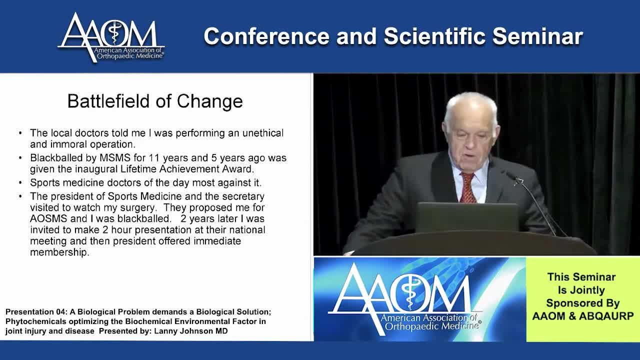 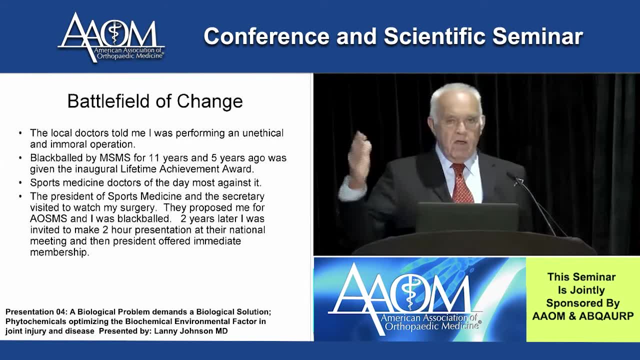 And I told you that the sports medicine doctors of the day were most against it. but the president and the secretary came to watch me because the hospital by that time had built a glass wall and put bleachers in it, so many people were coming. 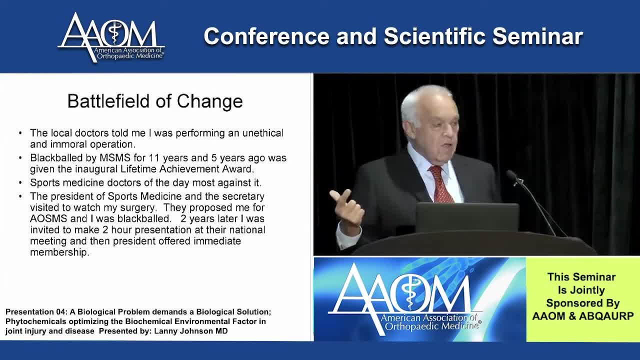 So the president put me up for the society, the secretary seconded me and I was blackballed and didn't get in, And so, two years later, they asked me if I'd make a two-hour presentation to their organization, the National Leading. 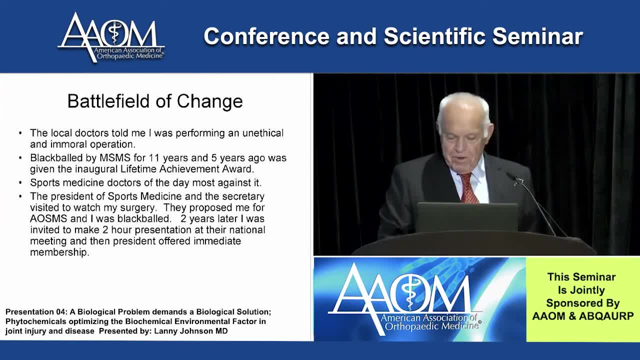 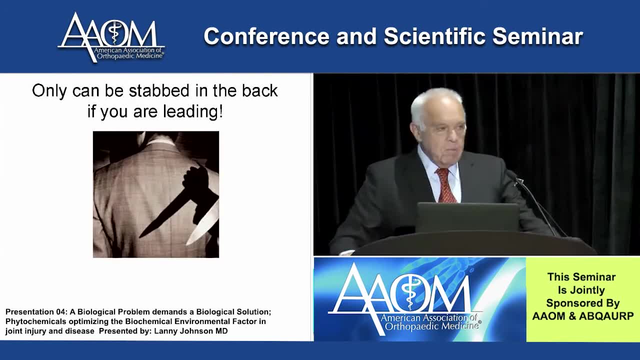 which I did, and they said: well, we'd like to offer you immediate membership. I said: fine, It doesn't matter that much to me. This will be helpful to all of you. You can only be stabbed in the back if you're leading. 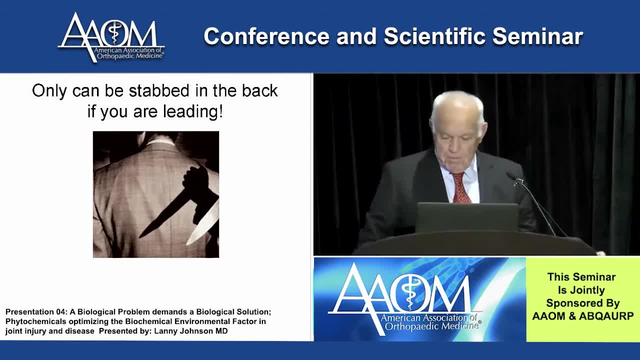 And so a lot of you may have experienced that, but if you're working on something, you've got to know that that's a potential. But here's the road to victory which I see this organization really has got to get more of. 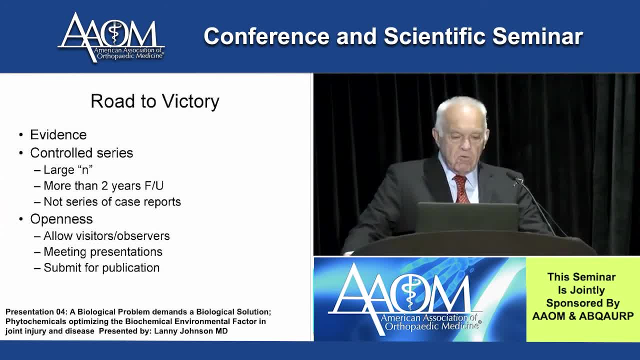 You've got to have evidence. You've got to have controlled series large enough in more than two years follow-up, not three weeks, and you can't have just a series of case reports. You've got to have a series of cases.